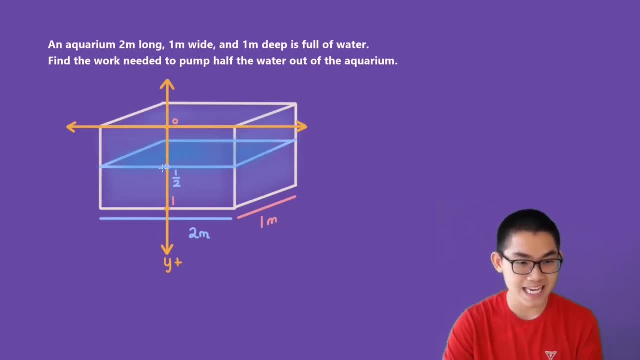 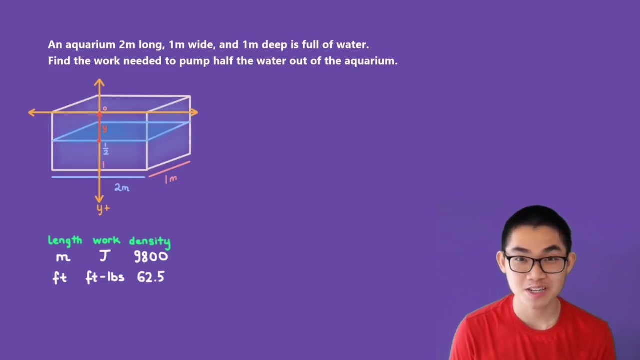 And what we're going to do is we are going to pull up each layer. We're going to pull this layer of water to the top. Last but not least, the distance that we're pulling each layer of water can be called y. We are now ready to solve this problem. 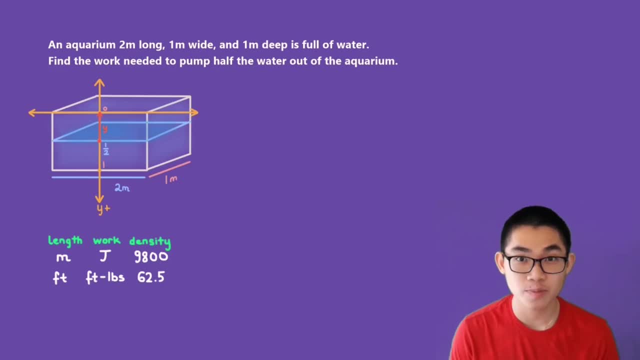 So what's the formula to calculate the amount of work to pump all the water out? Well, the work formula is going to be equal to W, which is work is equal to the integral from top to bottom, the bottom, And I'm going to show you how to find these numbers later. And here we have density. 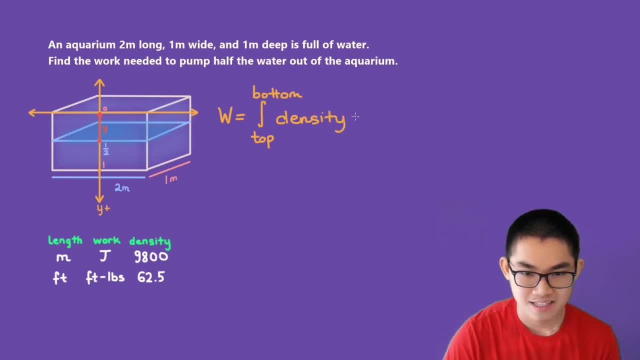 times the distance that we need to pull the layer of water to the top and times the area, And this area is basically the area of the layer of water. And then we have dy: What is the top and what is the bottom. Well, remember, we're pulling all the layers of water. 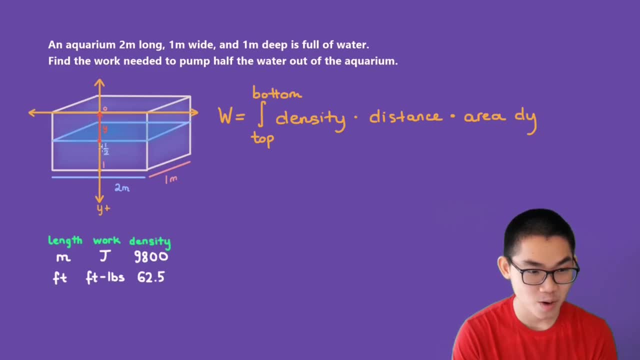 from the top, which is zero, and the bottom is one over two, And because of that, the bottom will be one over two right here. So this would be one over two and the top will simply be zero. Now, how about the density? Well, if the product is one over two, 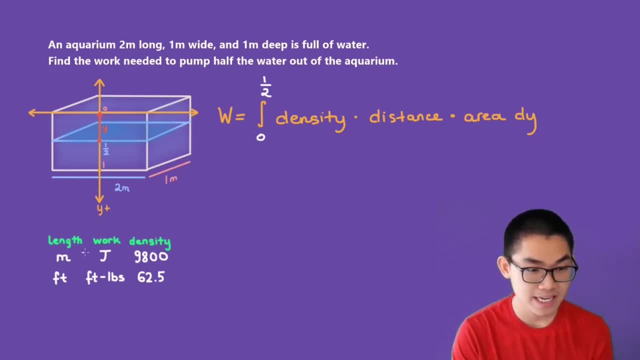 the problem is in meters. If they give you the length in meters, then the work will be in joules and the density will be 9,800.. So the density in this case will be 9,800.. If the problem gives you the length in feet, then the work will be feet pounds. 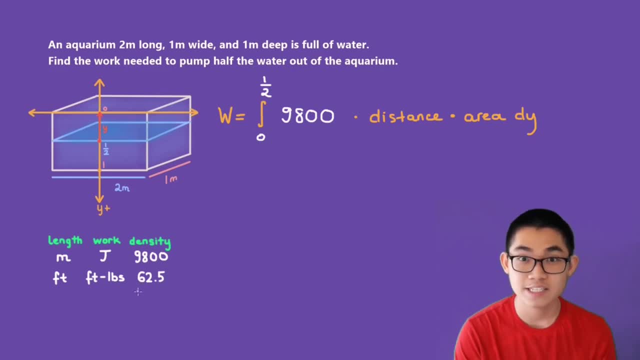 and the density will be a different number, So it will be 62.5.. The distance is the distance that we need to pull each layer to the top And, as mentioned before, that distance is simply y, So the distance here will simply be y. And then, how about the area? 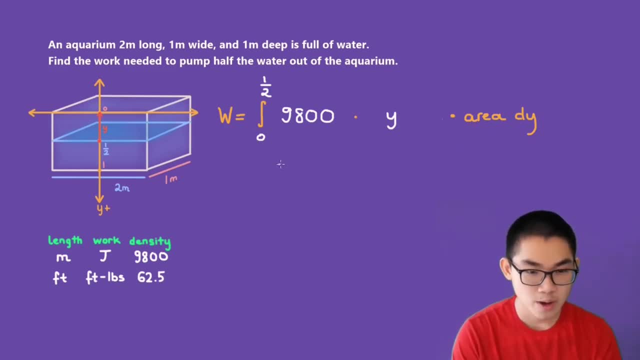 Well, what's the area of the layer of water? Well, you might learn before that the area of a rectangle- this is a rectangle- is equal to the base times the height, And we already know that the base is two meters. So the base is two, the height is one. So two times one gives you two. 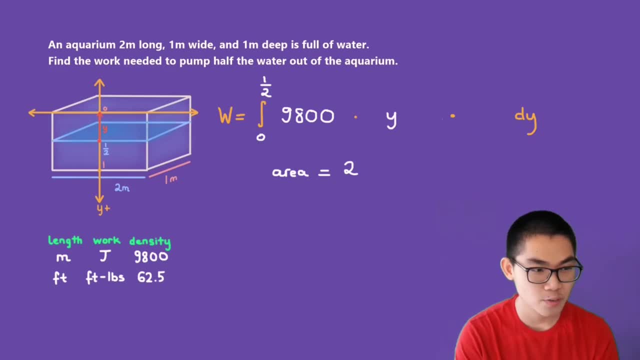 So the area is simply two meters square. I'm going to put in two for short, And let's get rid of this. Let's evaluate this integral. So 9,800 times two will give you 1,900.. So w or the work. 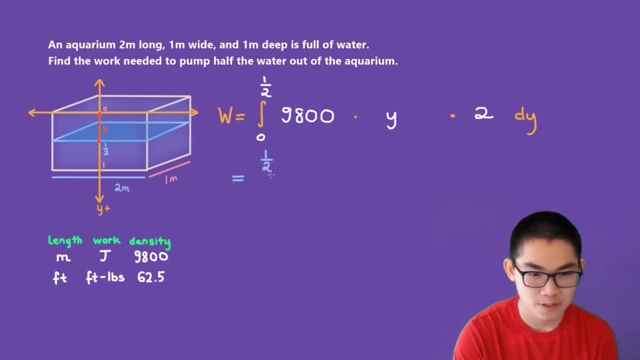 is equal to the integral from 0 to 1 over 2 of 19,600 times y times dy. So since this is a constant, we can move it outside of the integral. So we get 19,600 times the integral from 1 over 2.. And here is 0. y. this is: 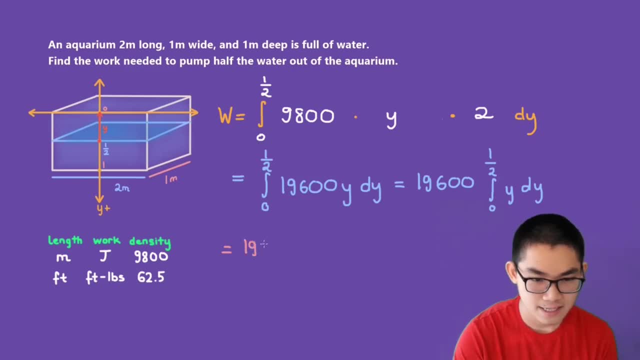 the same as 19,600.. Times the antiderivative of y, which is just 1 over 2 times y, to the power of 2.. And we have 0 and 1 over 2 at the top. This is the same as 19,600 times 1 over 2 times 1 over 2 to the power. 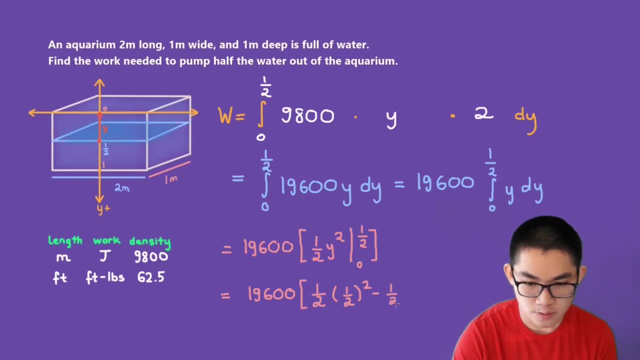 of 2.. Minus 1 over 2 times 0 to the power of 2.. Let's close that bracket Now. 1 by 2 to the power of two is 1 over 4.. And 1 over 4 times 1 over 2 gives you 1 over 8.. 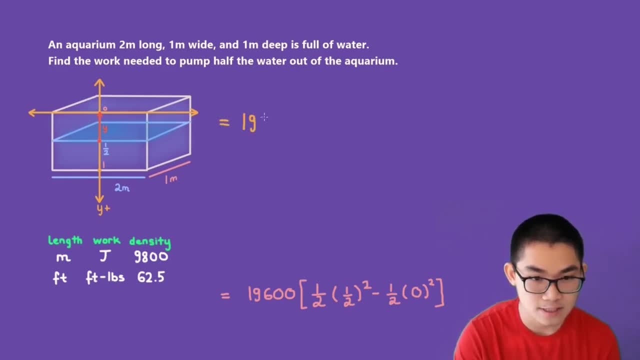 Now this is equal to 19,600 times 1 over 8, and this will simply give you 0,. so minus 0, and now 19,600, times 1 over 8 will give you 2450, and that's it. that is the answer and the. 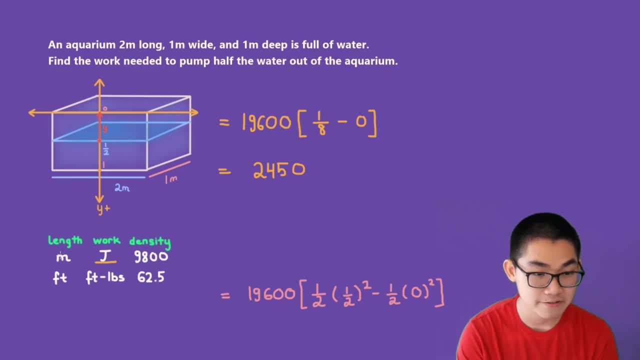 unit will be duels, remember, because the length they've given us its meters, so the answer will be 2450 duels. so this, right here, is the answer to this question and the amount of work that it takes to pump half the water out of the aquarium. we're gonna be doing some more. 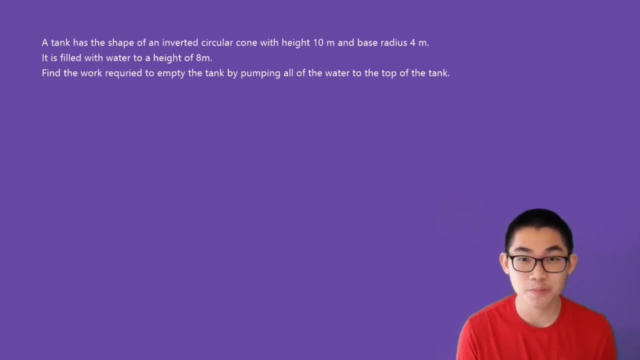 practice problems with calculating the amount of work to pump the water out of a tank. so this problem says a tank has the shape of an inverted circular cone with a height of 10 meters and a base radius of 4 meters. it is filled with water to a height of 8 meters and we have to find the work required. 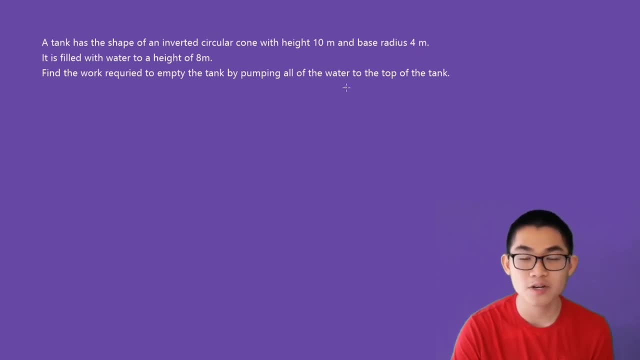 to pump the water out of the tank, to empty the tank by pumping all of the water to the top of the tank. so the first thing we have to do is draw out our diagram. so here is our circular inverted cone. it has a height of 10 meters and we also know that the base 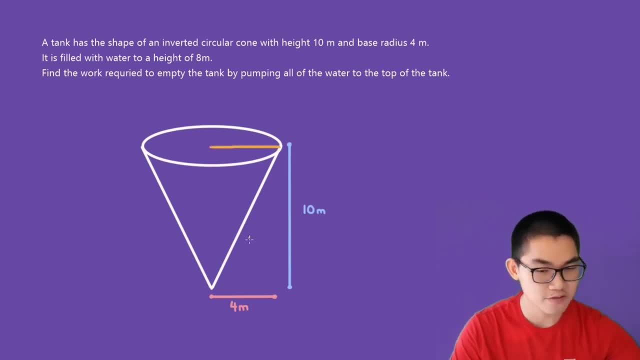 radius, or the radius from here here, so that radius is the same as 4 meters. the second step is to place our x and y axis. so remember, you have to place the x axis at the top of the shape and you have the y axis running down, like this. 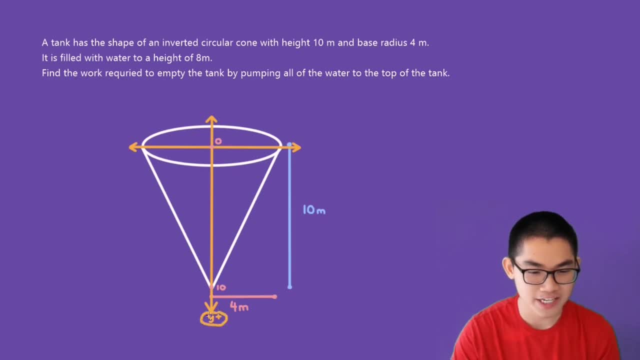 where the y direction, a positive y direction, is pointing downwards. so this point will be considered 0, or the origin, and this point will be 10, because the height from here to here is 10 meters. so the point here it will be n. we know that. 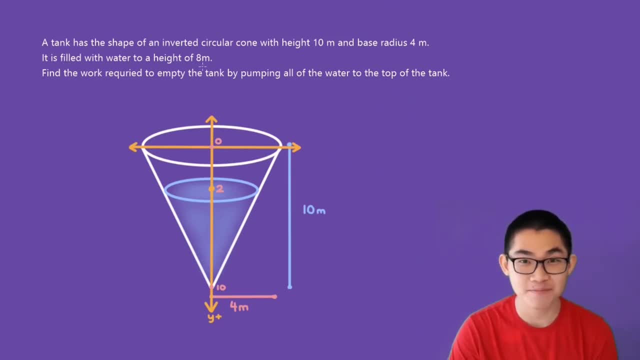 the tank is filled with water to the height of 8 meters, and 8 meters that would be from here to here, right? so this means that this point will be 2, because 2 to 10 is 8 meters. that's the difference between this distance. so that's why this point will be 2, the question asked us to 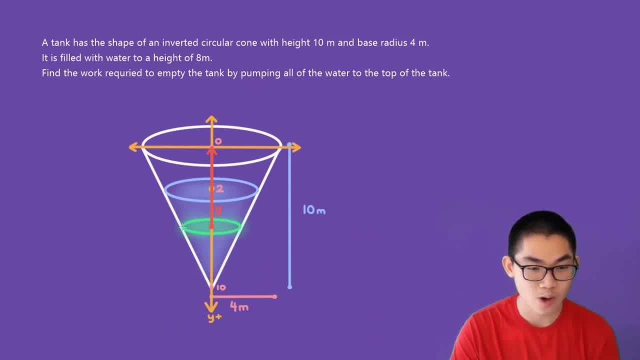 empty the tank, which means that we're going to pull out all of the layers of water. so there are many, many, many layers of water between 2 and 10, and let's say this is just one layer of water- water. I'm not going to draw out all the layers of water or else it's going to look very messy. 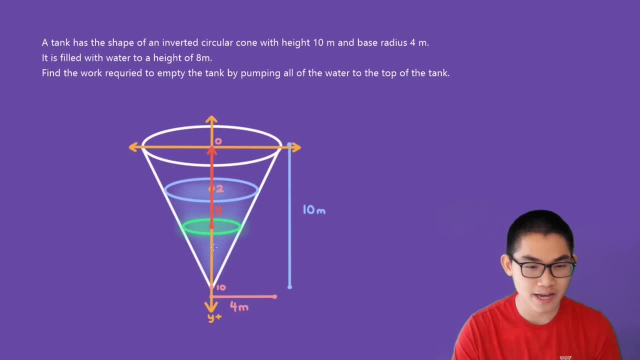 But basically the idea is that for every single layer of water like this one, we're going to pull it to the top of the tank, right, And we're going to do this for every single layer of water, And that's basically how we empty this tank. So the distance that we pull this layer of water to the 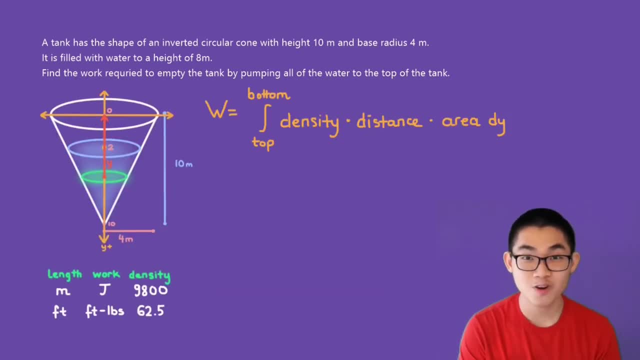 top will be considered y, So the formula that you want to use is w, for the work is equal to the integral, from the top to the bottom, of density times, distance times, area, e, y. So what's the top and what's the bottom? Well, the bottom is right here and the top is right here, because we want to 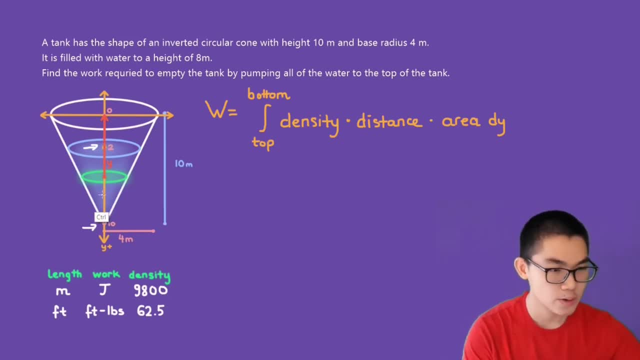 empty the tank from 2 to 10,, right, So the bottom will be 10. And the top will be 2.. How about the density? Well, if you look at this table, the problem has given us the length in meters, so the work will be in joules and the density will. 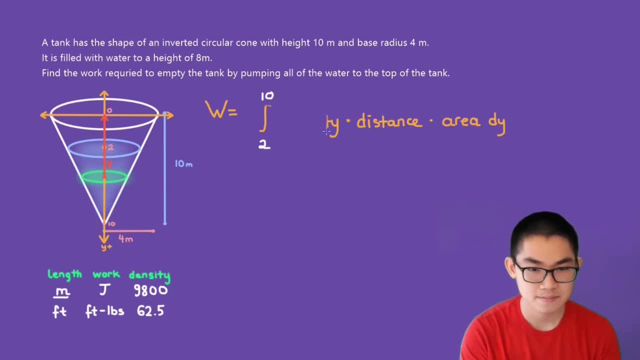 be 9,800.. The distance is y, as mentioned before. How about the area of the layer of water? So if you look here, this is a circle right, Which means that the area of that layer of water is equal to pi times the radius to the power of 2.. So this is pi times the radius. 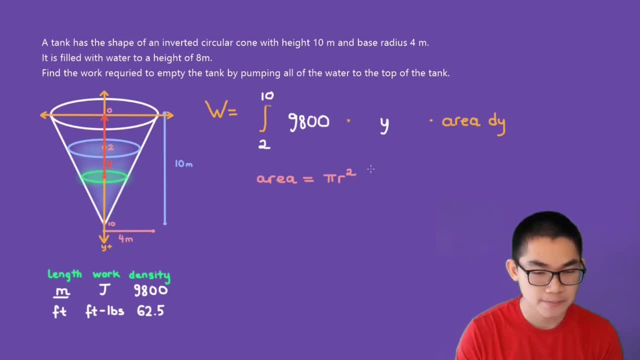 to the power of 2.. So this is pi times the radius to the power of 2.. So this is pi times the radius to the power of 2.. And the radius is from here to here. That's the radius, And the distance from here to here is x because it is horizontal. So instead of r I'm going. 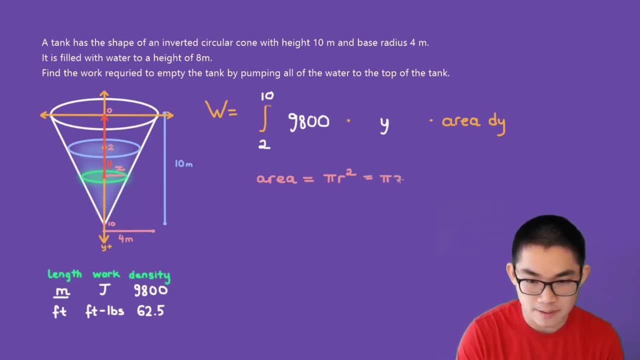 to write it as x. So this is equal to pi times x, to the power of 2.. Since the equation, or rather the formula, is dy, we have to change all of our variables into y. So let me show you how to do that. 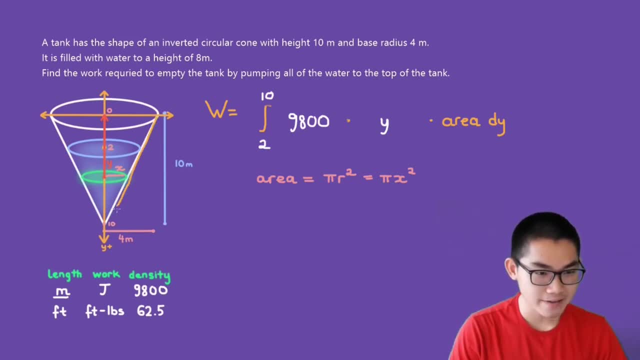 Now, if you look here, this is a line. right, That looks like a line, So you can use what you learned in high school to find the value of y instead of x. Now, this point, right here, this point will be 4, 0.. Why is it 4, 0? Because the distance from here to here is 4, which. 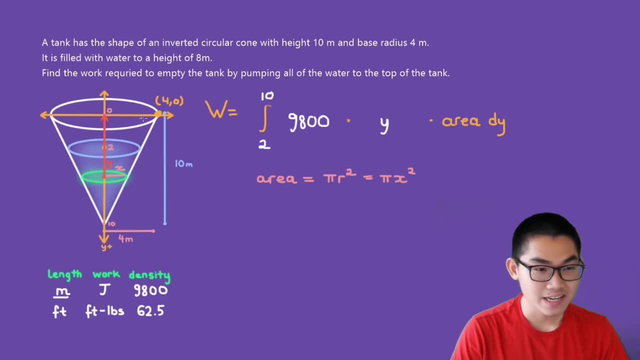 means the distance from here to here is also 4.. So this is 4, the height is 0. And how about this point right here? Well, that point is 0, 10, because the x value is 0 at the origin and the y value is 10.. 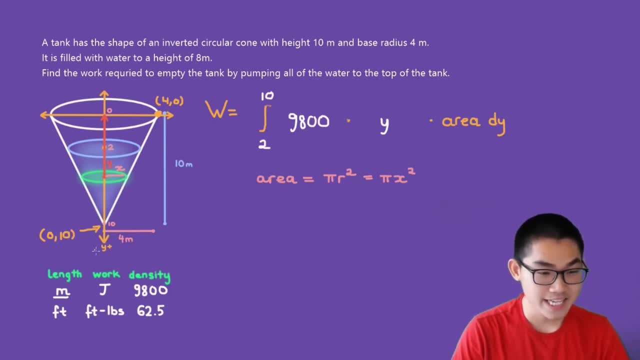 And notice that 10 is a positive number because we're saying that this direction is positive. You know, it's better to work with positive numbers than numbers that are below 0, right Now, we can use these points to find the slope formula, And these two points are, let me 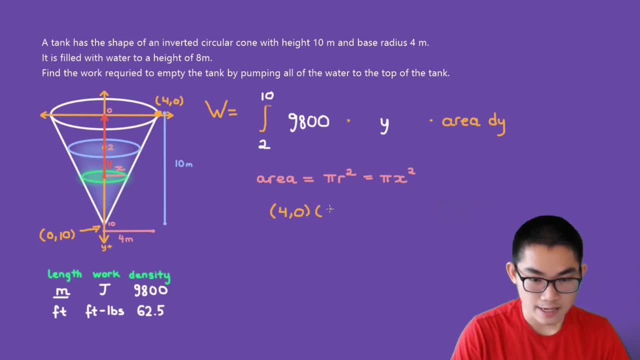 write them out here: 4, 0. And 0, 10.. So the slope, the slope m, is equal to 10 minus 0, and 0 minus 4.. 10 minus 0 is equal to 10.. 0 minus 4 is negative 4.. We can simplify this into negative 5 over 2.. Now 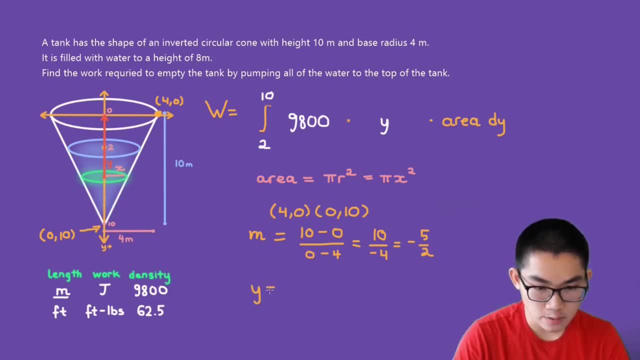 our equation will be: y is equal to negative 5.. And we're going to substitute this point. let's say this point right here. we're going to substitute this point into our equation. So we substitute: y is equal to 10.. And then 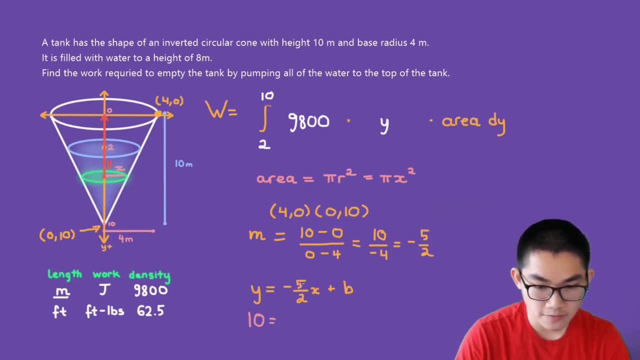 x is 0. So 0 times 5 over 2 will be 0, itself plus b. This means that b is equal to 10, right b is equal to 10.. So we're going to delete the b and replace it with number 10.. 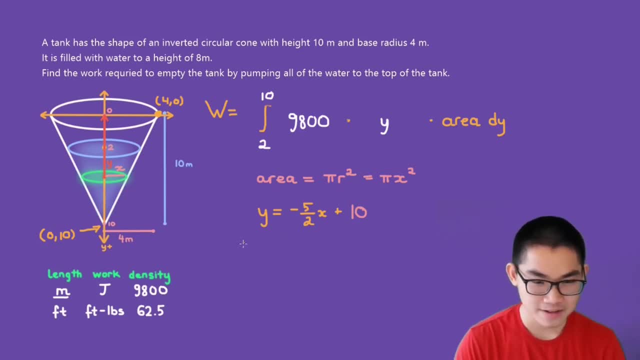 Let's solve for x. So I'm going to add to both sides, we get y. plus 5 over 2, x is equal to 10.. We subtract both sides by y, we get 5, oops, let me write a little bit below that. So 5 over 2 x is: 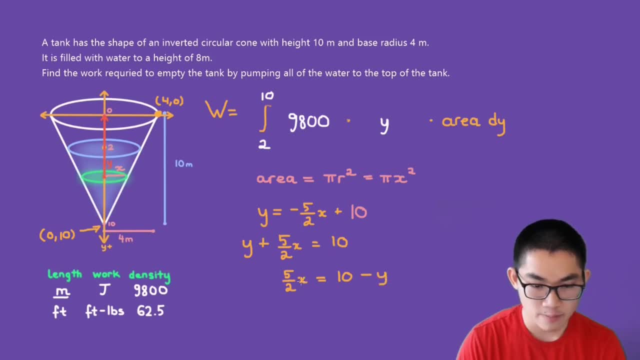 equal to 10. minus y. And if we multiply both sides by the reciprocal or 205, we get x is equal to2 over 5 times 10, minus y. So that's how you find x. So we're ready to put it into. 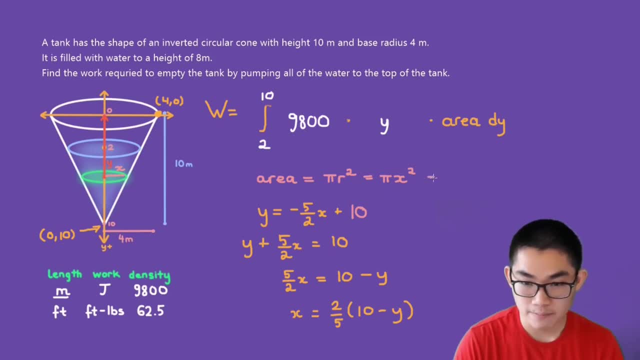 our area equation we're going to get pi times x and x is equal to this right. So we just put in 2 over 5. times n minus y, and now notice that here is x to the power of 2. so don't forget the power of 2 up. 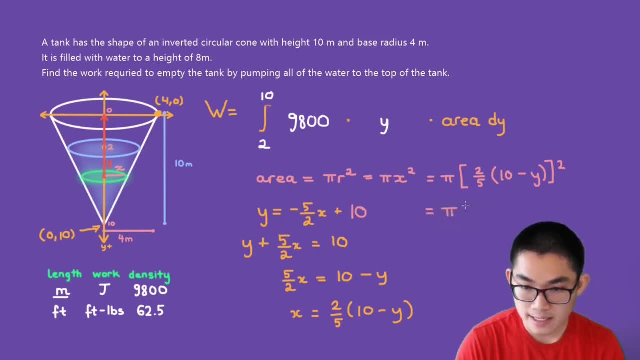 here. let's simplify this. so we get pi times 4 over 25, 4 over 25 times n minus y to the power of 2. let's evaluate this integral. so what is 9800 times 4 over 25? i put into the calculator: 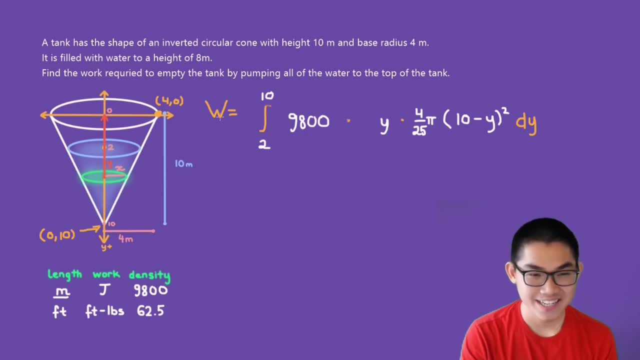 and it gives me 1568. so this is equal to the integral from 2 to 10. this is 1568, and don't forget the pi over here. so this is pi times y times n minus y, to the power of 4 over 25. 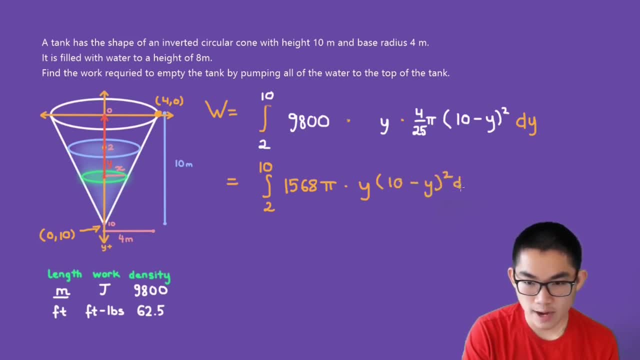 minus y to the power of 2 dy. And since this is just a constant, let's go ahead and move it outside of the integral. So we get 1568 times pi, times the integral from 2 to 10.. And here we have y times 10 minus y to the power of 2 dy. Now, what is 10 minus y to the 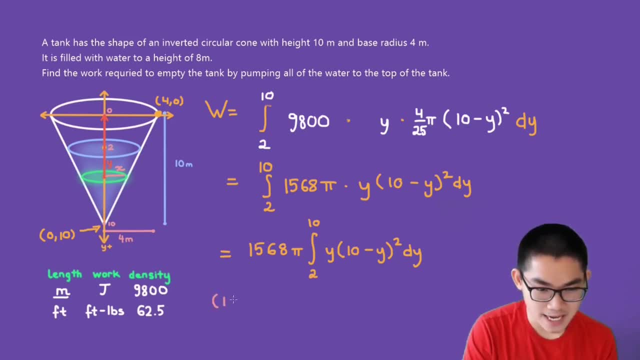 power of 2?? Let's find out. So we have 10 minus y to the power of 2.. This is the same as 100 minus 20y plus y to the power of 2.. So let's go ahead and put this into our integral. 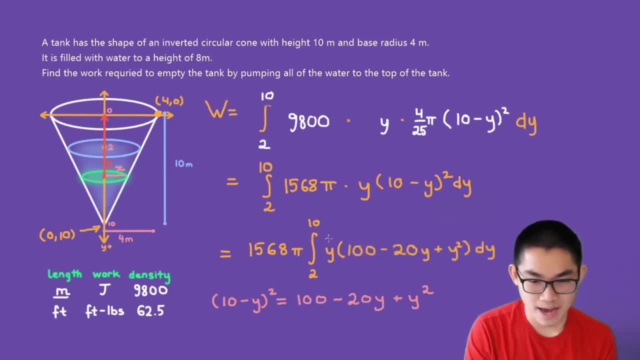 And if you look here, we can also simplify this by multiplying this whole expression with y. So we're going to multiply each term with y. We're going to get 100y minus 20y to the power of 2 plus y to the. 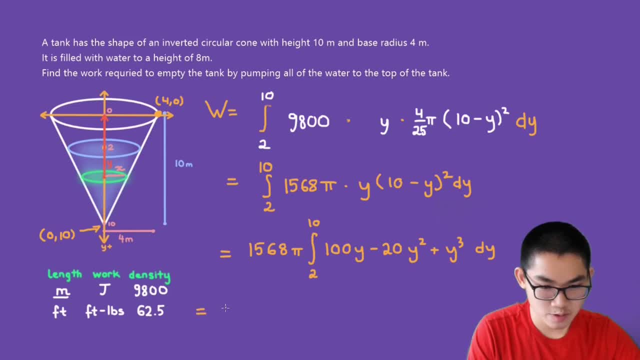 power of 3.. This is equal to 1568 times pi, times the antiderivative of 100y. So the antiderivative of y, as we know, is 1 over 2.. So if we multiply this together we are going to get 50y2 minus the antiderivative of 20y. 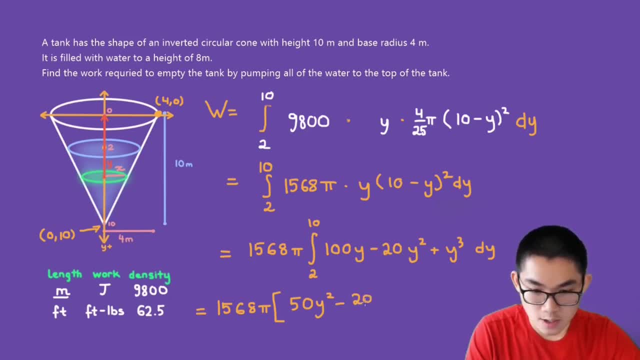 to the power of 2.. Well, that's just going to give you 20 over 3 times y to the power of 3.. And the antiderivative of this one is pretty easy. It is just 1 over 4 times y to. 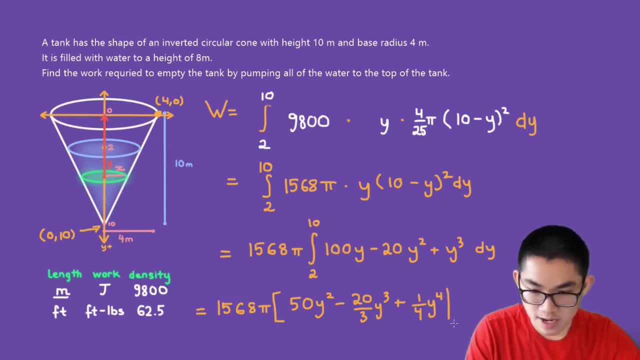 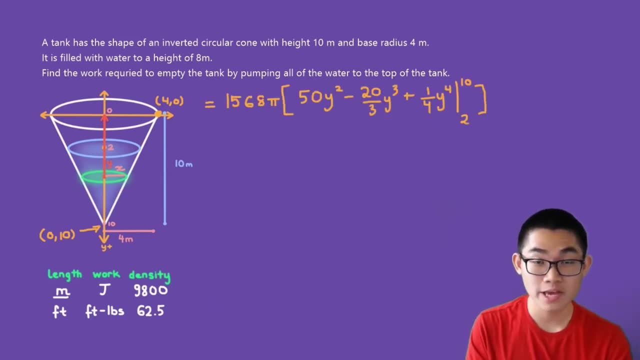 the power of 4. And we have the limit. It goes from 2 to 10.. So we're going to multiply 2 to 10. And we can go ahead and close that bracket right there. So it is pretty simple from here, And all you need to do is substitute in these numbers. 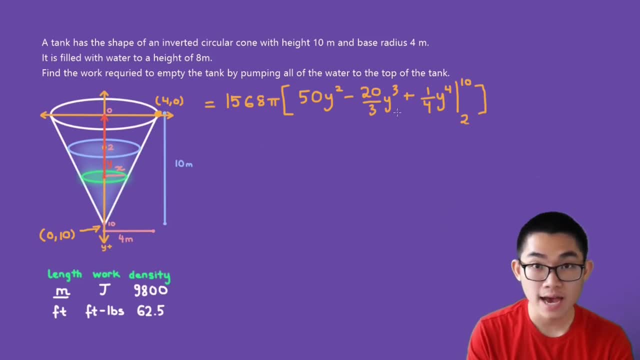 for the upper bound and lower bound into the equation And after you simplify it, you should get 1568 times pi times 2048 divided by 3.. So that's what I have. After I put this into my calculator, I get 3362827.797.. And this is approximately 3.4 times 10 to the power of 6 joules, because 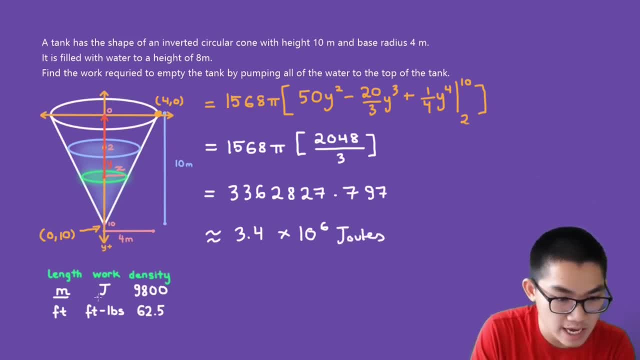 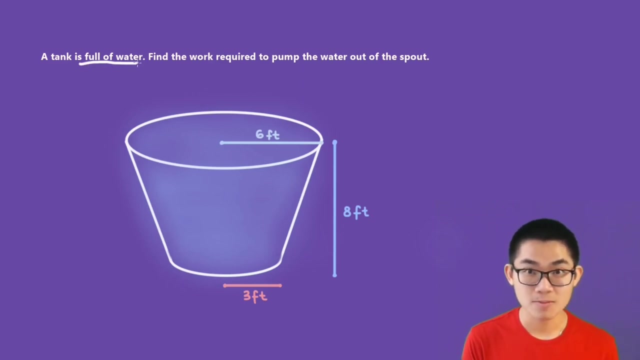 remember, the unit here is joules, according to the table, And so this is the same answer as the textbook. So this number right here is the amount of work that it takes to empty this entire tank. So we're given a tank that is full of water And the problem wants us. 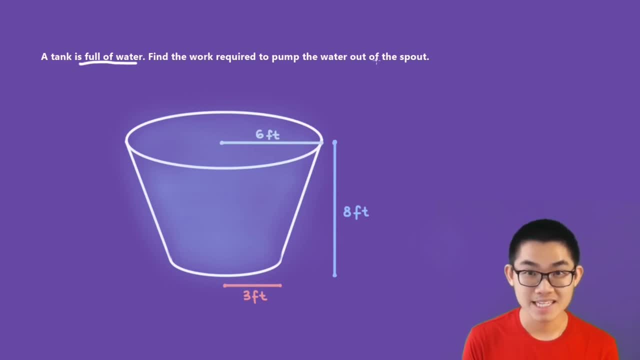 to calculate the amount of work required to empty this tank, The first step is to put the x and y axis looking like this, where this direction is the positive direction for the y axis. So we know that our tank is 8 feet tall because 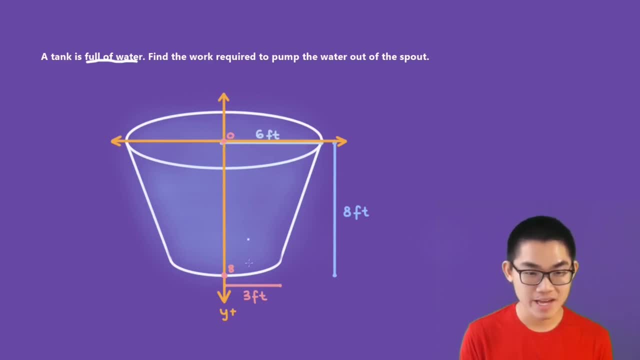 the height is 8 feet, So that's why this point is 0, and this point will be positive 8.. And we also know that the radius of the top circle is 6 feet, so the distance from here to here is 6 feet And the distance from here to here is 3 feet. To empty this tank, all we have. 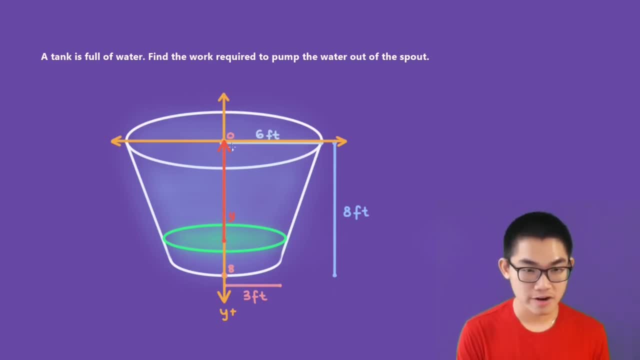 to do is move every layer of water like this one. So there are many layers of water here, So we're going to move each layer of water to the top of the tank, And the distance from the origin to our layer of water is called y. 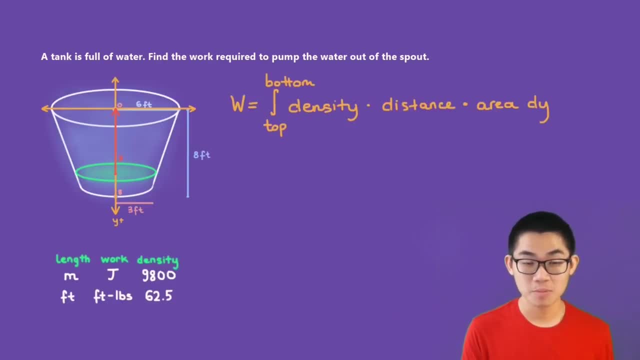 To calculate the work, all you have to do is use this formula: w, or. the work is equal to the integral, from the top to the bottom, of density, times, distance times, area. So what is the top and what's the bottom? Well, as mentioned before, we want to empty. 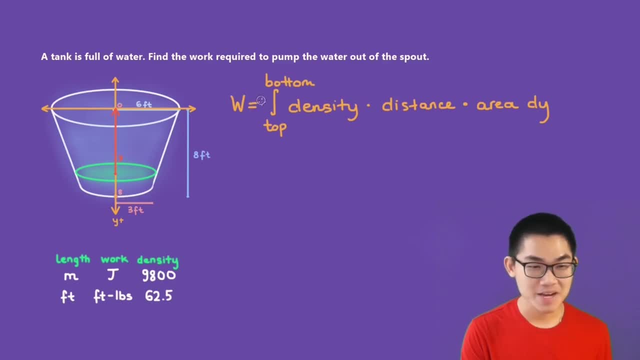 this tank from 0 to 8, right, So the bottom will be 8, and the top will be 0.. How about the density? Well, according to this table, if the tank is measured in feet- in which case it does- then we need to use the density. 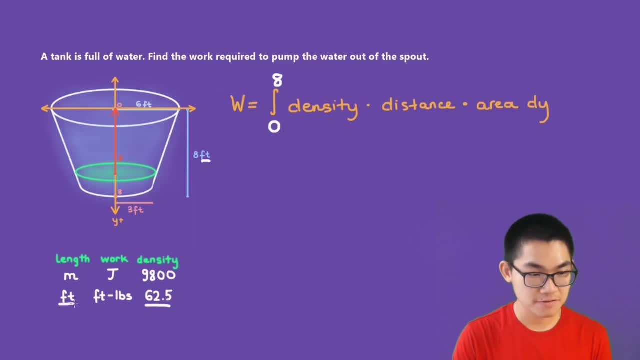 which is 62.5, because the length is in feet. The density will be 62.5.. The distance that we're pulling each layer of water is y, because we're pulling it to the top, So the distance will simply be y. Last but not least, we need to find the area. 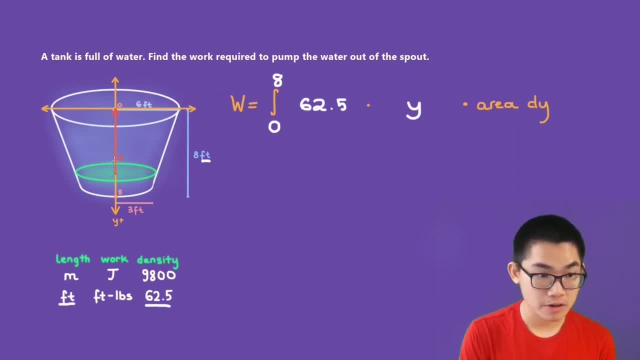 So this area is referring to our layer of water right here. So since our layer of water is a circle, the area of this layer of water is equal to pi times the radius to the power of 2.. And the radius from here to here is x. So instead of writing r, I'm going to write: 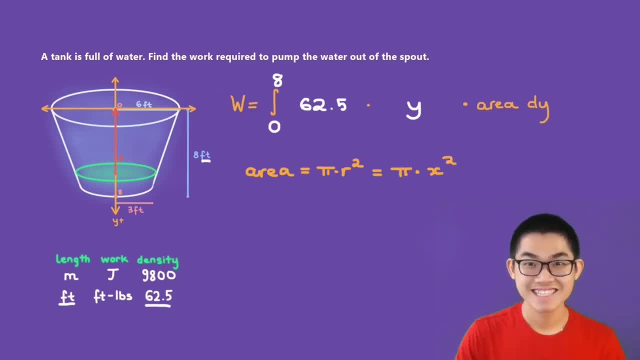 it in terms of x. Since our line is dy, we have to convert the x into the y, And let me show you how to do that. So if you look here, this is a line right, So you can use the formula of a line to find. 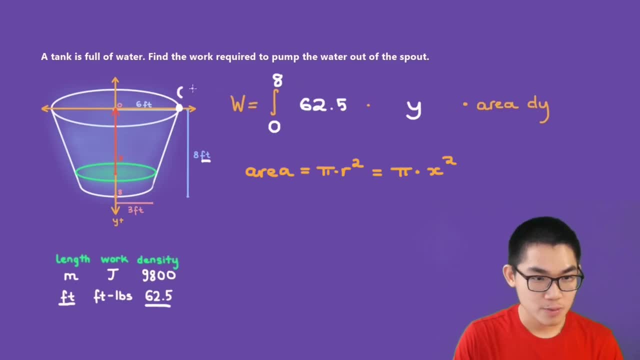 y. We know that this point right here will be 6, 0, because the distance from here to here is 6, right, And the height is 0, so therefore it will be 6, 0.. Now, how about on this line? How about this point right here? 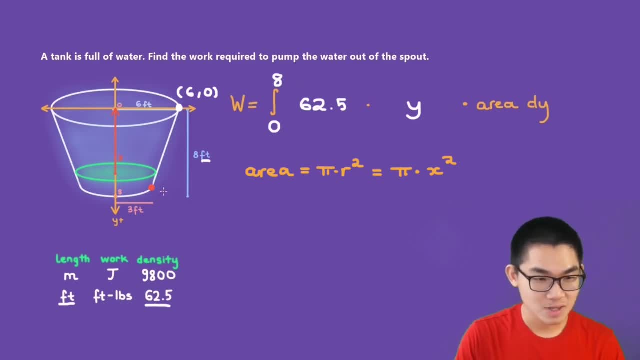 Well, this point will be 3, 8.. So this point will be 3, 8.. And why is it 3, 8?? Well, because the distance from here to here is 3, and the height is 8.. Now notice that 8 is a positive number. 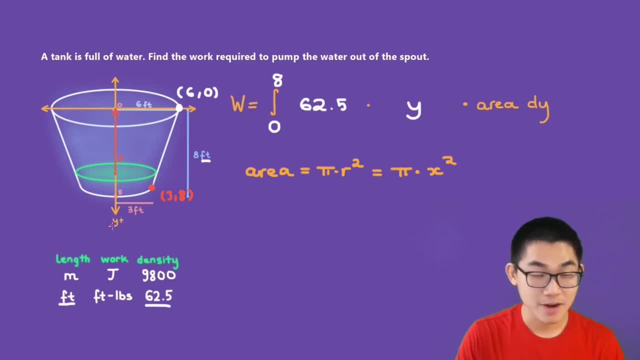 because we're saying that the positive y-direction is right here. So let's write out our two points. We have 6, 0, and we also have 3, 8.. The slope m will be the same as 8 minus 0, divided by 3 minus 6.. This is the same as 8, divided by. 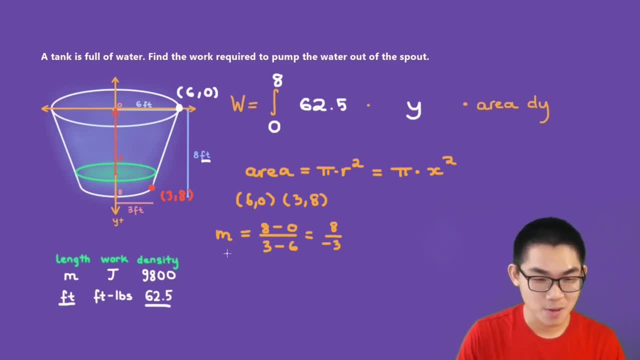 negative 3.. So putting this into our point-slope formula we get: y, which is the variable we're looking for, is equal to negative 8 over 3 times x plus b. Now all we have to do is substitute in one of these two points. Let's put in this one. 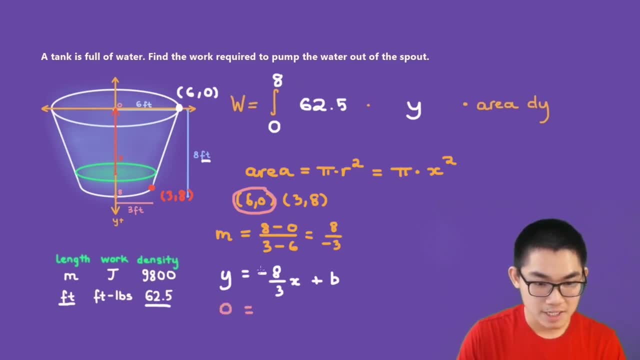 so y is equal to 0 and x is equal to 6, so this will be negative 8 over 3 times 6 plus b, and negative 8 over 3 times 6 is equal to negative 16.. so therefore, b is equal to 16.. and let's delete this b and write in 16.. 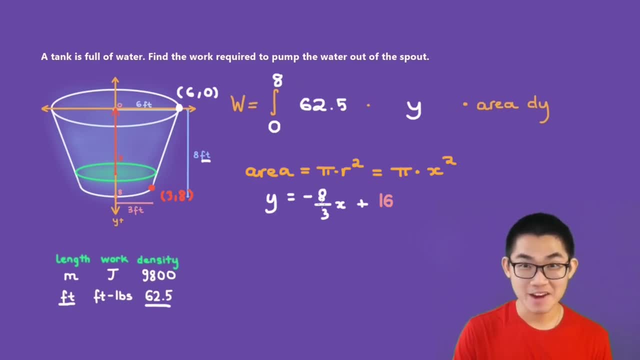 so here is our equation: y is equal to negative 8 over 3 times x plus 16.. now let's solve for x. we subtract both sides by 16, so we get: y minus 16 is equal to negative 8 over 3 x. and then we: 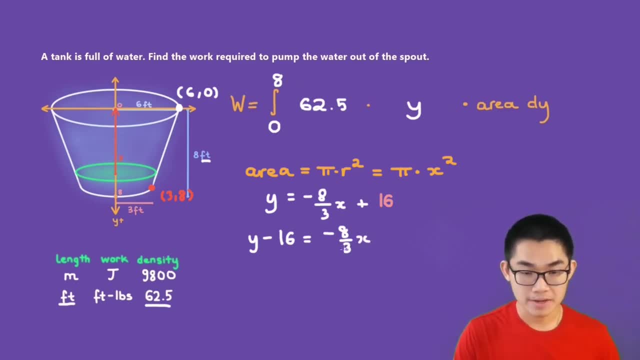 multiply both sides by negative 3 over 8, so we get: x is equal to negative 3 over 8 times y minus 16.. so we finally found x and we can substitute this right here into our x squared in order to find the area. so the area is equal to pi times x, to the power of 2, and we know that x is equal to this. 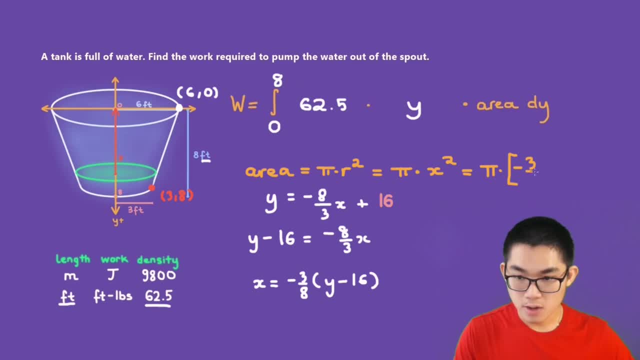 expression right here which is negative: 3 over 8 times y minus 16- close the bracket- and to the power of 2.. this is equal to pi times 9 over 64, so 9 over 64 times y minus 16 to the power of 2.. 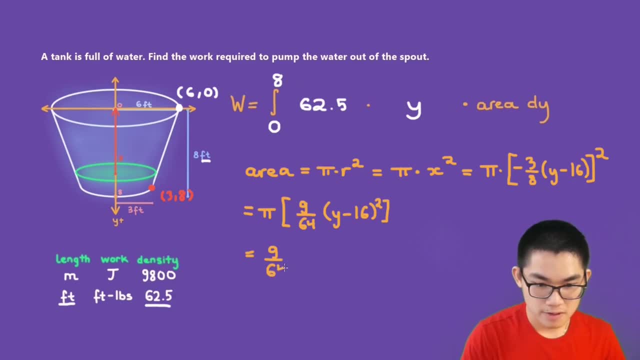 and this is the same as 9 over 64 times pi, times y minus 16, to the power of 2.. now that we found the area, let's go ahead and put it into our formula. we are almost done. the last step is to evaluate this integral. so this is equal to the integral. 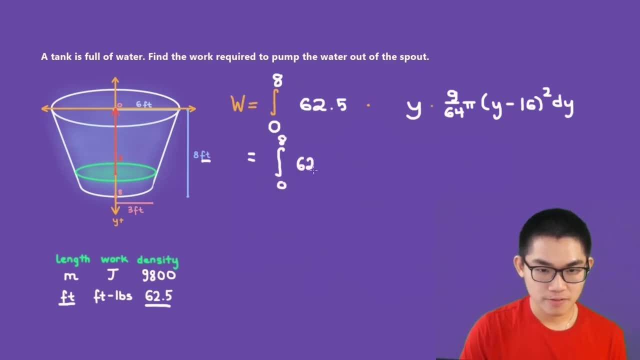 from 0 to 8 times 62.5 times 9, over 64 pi times y times y minus 16, to the power of 2 dy. and since these numbers right here are constants, we can move it outside of the integral as well. so 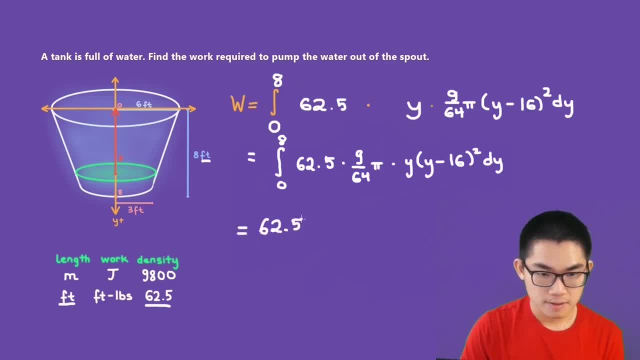 this is equal to 62.5 times 9 over 64 pi, times the integral from 0 to 8, times y, times y minus 16 to the power of 2 dy. now, what is y minus 16 to the power of 2? 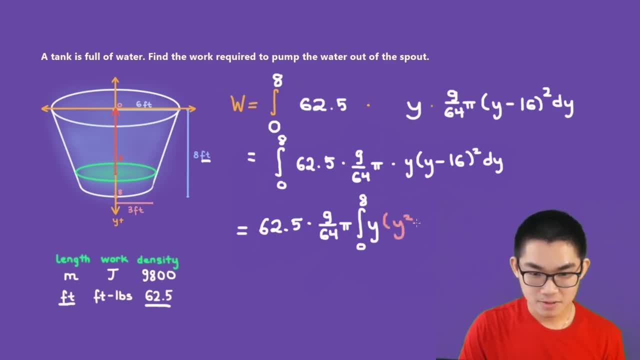 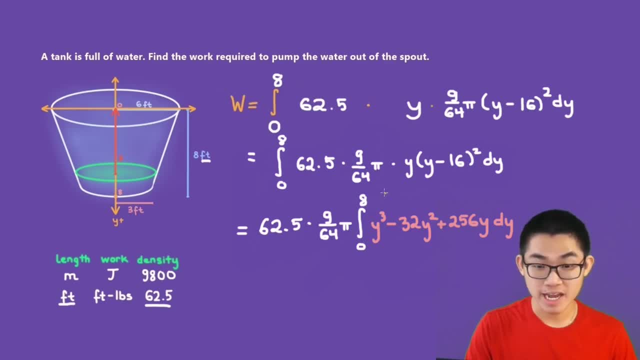 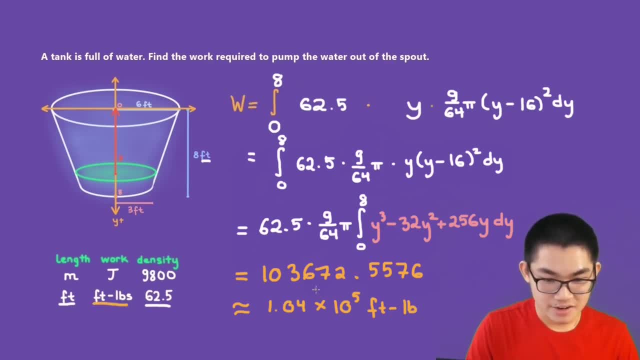 pound, because the unit here is feet pound according to our table, and so this pound according to our table, and so this pound according to our table, and so this here is the answer, and also the amount here is the answer, and also the amount here is the answer, and also the amount of work that it takes to empty this tank. 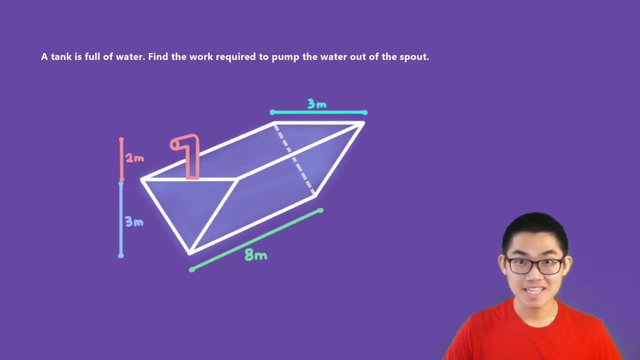 of work that it takes to empty this tank of work that it takes to empty this tank. in this video, i'm going to show you how. in this video, i'm going to show you how. in this video, i'm going to show you how to calculate the amount of work that it. 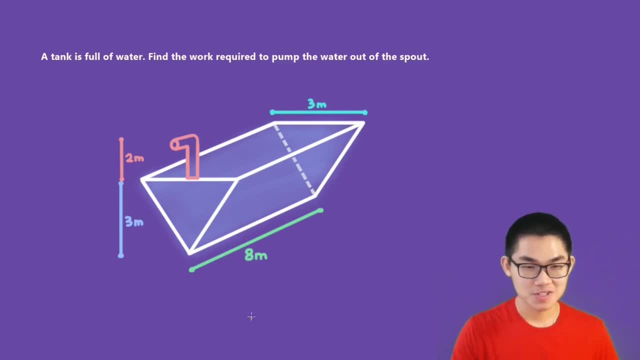 to calculate the amount of work that it. to calculate the amount of work that it takes to empty a tank full of water. takes to empty a tank full of water takes to empty a tank full of water. so we're given this tank it is full of. so we're given this tank it is full of. 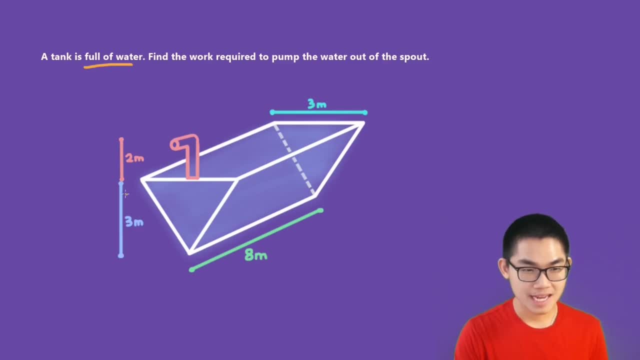 so we're given this tank. it is full of. we know that the length of this tank is. we know that the length of this tank is. we know that the length of this tank is eight meters, eight meters, eight meters, and the height of this tank is three. 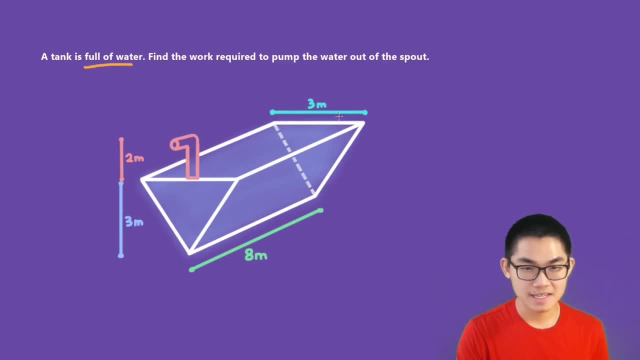 and the height of this tank is three, and the height of this tank is three meters, meters, meters, and the width of this tank is also three, and the width of this tank is also three, and the width of this tank is also three meters, meters, meters. and then we have a spout like this: it's: 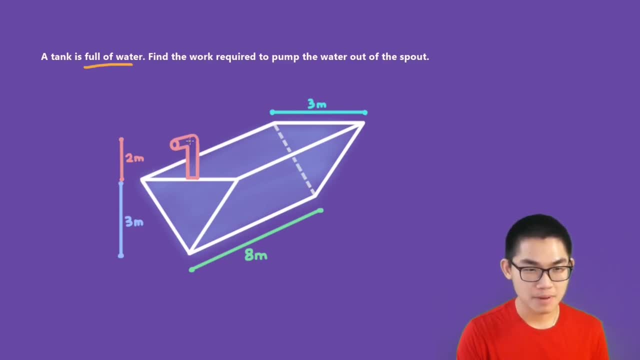 and then we have a spout like this: it's. and then we have a spout like this: it's two meters, and we have to move all of two meters, and we have to move all of two meters and we have to move all of the water and pump it outside of the. 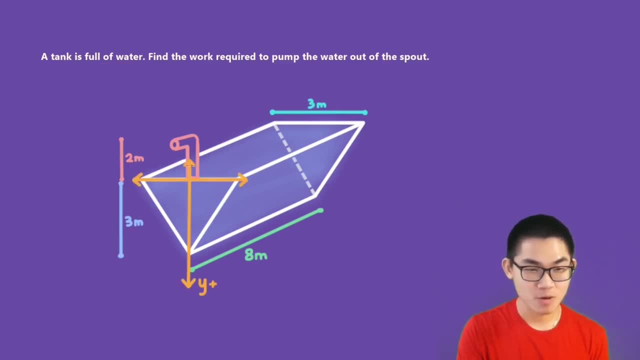 the water and pump it outside of the the water and pump it outside of the spout, spout, spout. the first step is to place an x and y. the first step is to place an x and y. the first step is to place an x and y axis. 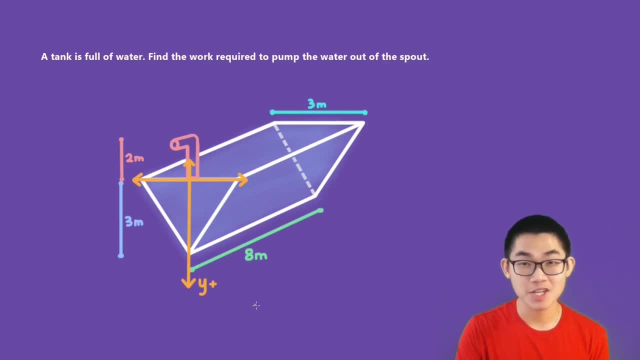 axis, axis with the y-axis pointing downwards, this with the y-axis pointing downwards, this with the y-axis pointing downwards, this way. so this is the positive direction way, so this is the positive direction way, so this is the positive direction. the second step is to draw our layer of. 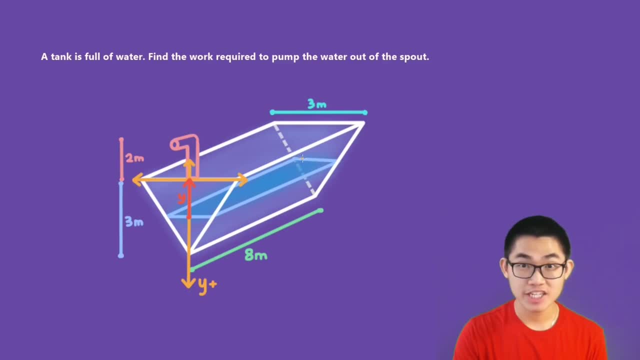 the second step is to draw our layer of. the second step is to draw our layer of water, water, water. so this is one layer of water, and you so this is one layer of water, and you so this is one layer of water, and you can imagine that there are many, many. 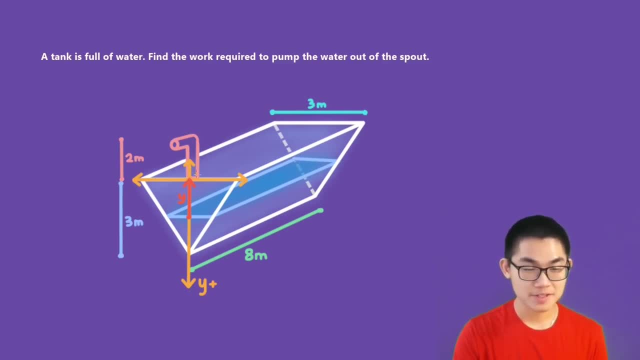 can imagine that there are many. many can imagine that there are many, many layers of water, layers of water from here to here, right so, in order to from here to here, right so, in order to from here to here, right so, in order to empty this tank, we need to move each. 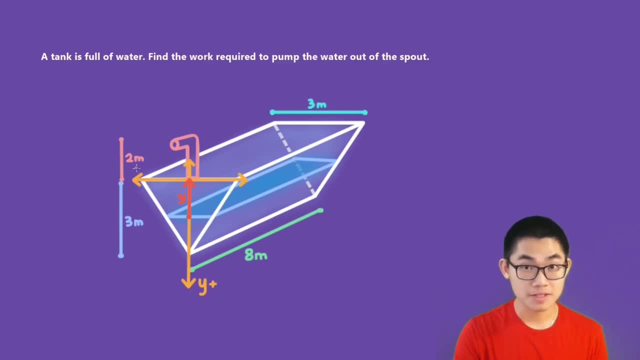 empty this tank. we need to move each empty this tank. we need to move each layer of water, like this one to the top layer of water, like this one to the top layer of water, like this one to the top and out of the spout and out of the spout. 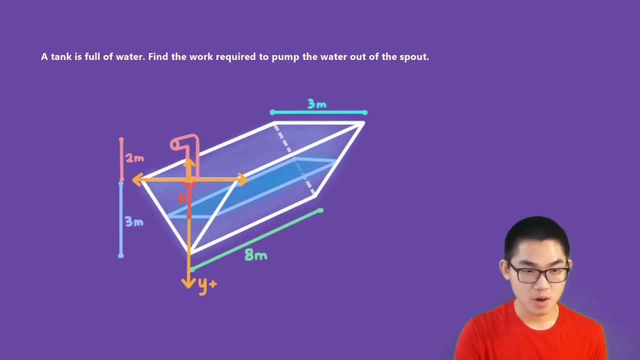 and out of the spout. and so the distance from the origin right, and so the distance from the origin right, and so the distance from the origin right, here, the origin of the axis, here the origin of the axis, here, the origin of the axis to our layer of water, this distance can. 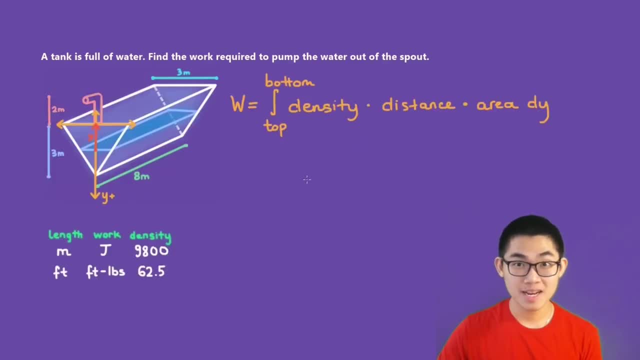 to our layer of water. this distance can to our layer of water, this distance can be considered, be considered, be considered as y. so the formula to calculate the as y. so the formula to calculate the as y, so the formula to calculate the amount of work to pump the water out of. 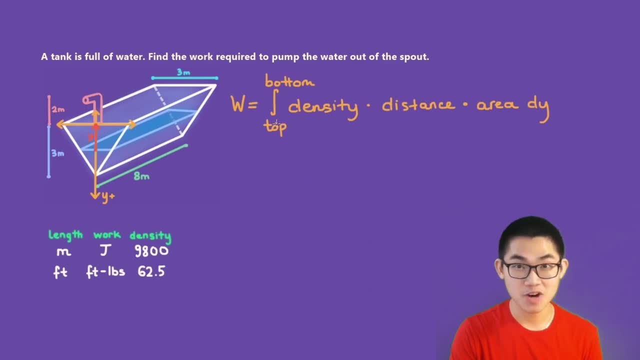 amount of work to pump the water out. of. amount of work to pump the water out of a tank is w is equal to the integral. a tank is w is equal to the integral. a tank is w is equal to the integral from the top to the bottom of density. 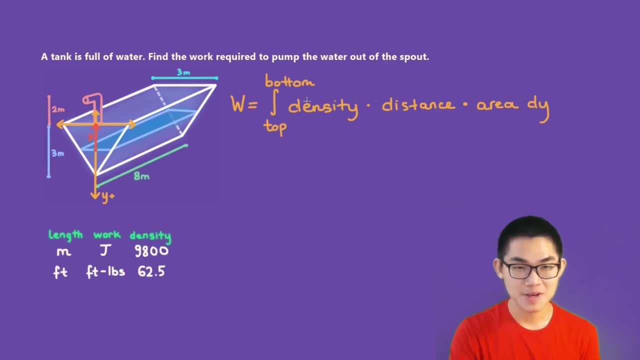 from the top to the bottom of density, from the top to the bottom of density, times, distance times, area times. distance times, area times, distance times, area. so, first of all, what is the bottom? and so, first of all, what is the bottom? and so, first of all, what is the bottom and what's the top? 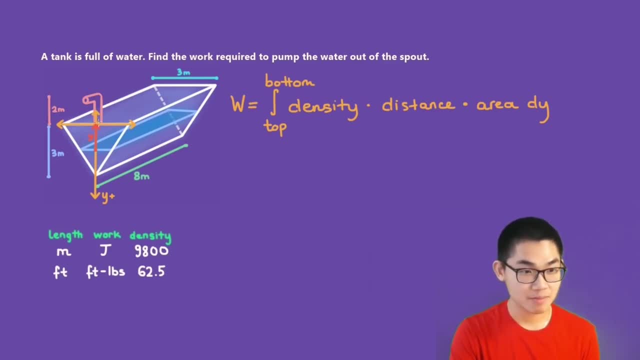 what's the top? what's the top? well, as mentioned before, we want to well, as mentioned before, we want to well, as mentioned before, we want to empty the tank from the top, which is empty, the tank from the top, which is empty, the tank from the top, which is here, to the bottom, which is here. 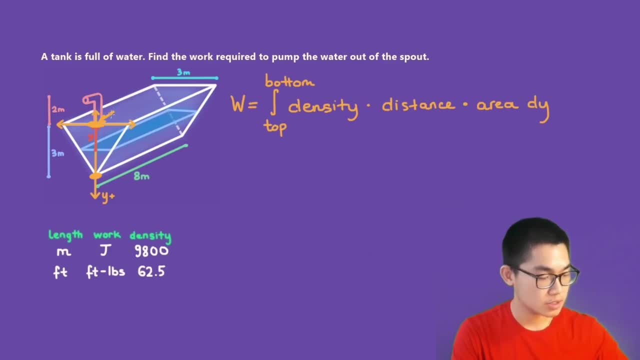 here to the bottom, which is here here to the bottom, which is here, right. so the top right here is the origin, right, so the top right here is the origin, right so the top right here is the origin, which is zero, so this point is zero. the, which is zero, so this point is zero, the. 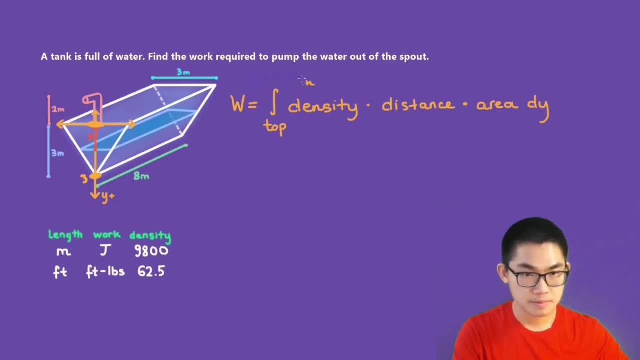 which is zero. so this point is zero. the origin and this point is three: how about the density? how about the density? how about the density? well, if we look at the table, we're given. well, if we look at the table, we're given. well, if we look at the table, we're given the length in meters. so the work will be. 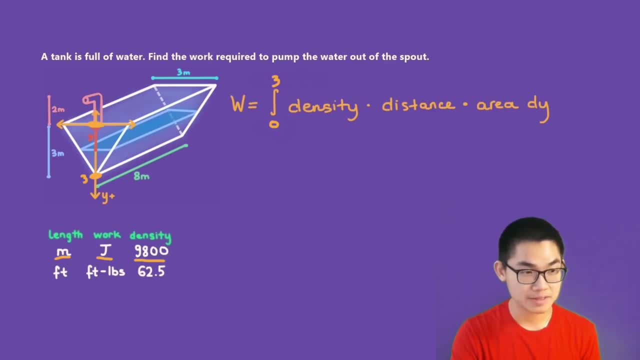 the length in meters. so the work will be the length in meters. so the work will be in joules and our density is 9800 in joules and our density is 9800 in joules and our density is 9800. what about the distance? 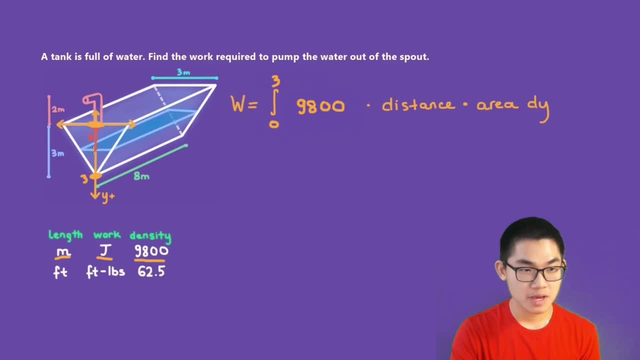 what about the distance? what about the distance? well, the distance to pump it to the top. well, the distance to pump it to the top. well, the distance to pump it to the top is y right the distance we're pulling is y right, the distance we're pulling. 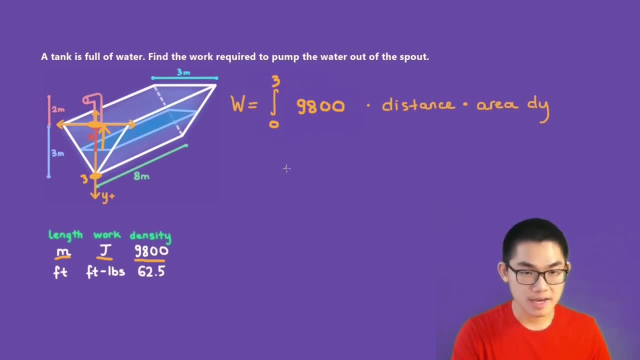 is y, right the distance we're pulling: the layer of water to the top, the layer of water to the top, the layer of water to the top. right there is y, but then we also have right, there is y, but then we also have right, there is y, but then we also have to pull it. 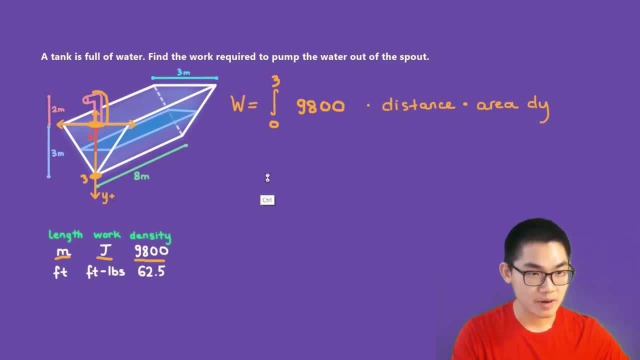 to pull it, to pull it outside of the spout. we have to pull it outside of the spout. we have to pull it outside of the spout. we have to pull it outside of the spout as well, outside of the spout as well, outside of the spout as well. so the distance is just y. 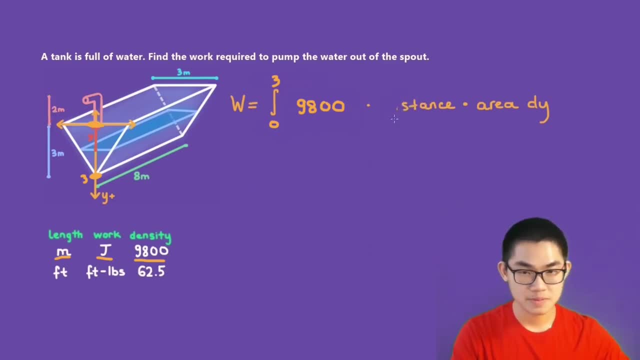 so the distance is just y. so the distance is just y plus two. last but not least, we need to find the last but not least. we need to find the last but not least. we need to find the area, area, area. so let me show you how to do that. 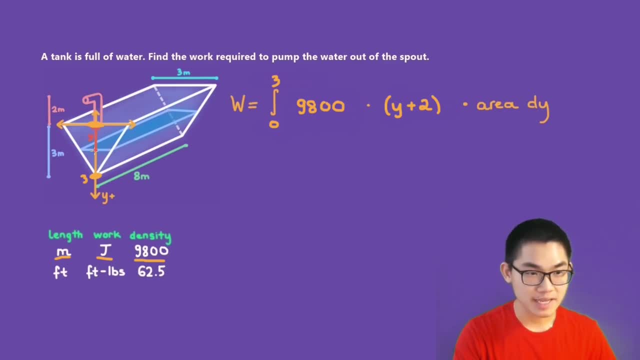 so let me show you how to do that. so let me show you how to do that now, the area of this layer of water. this, now the area of this layer of water. this now the area of this layer of water. this is a rectangle, so the area. 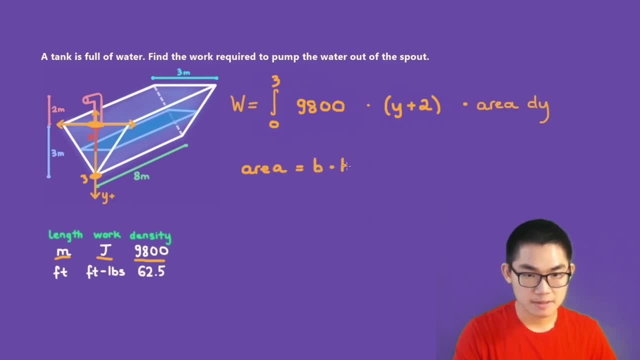 is a rectangle, so the area is a rectangle, so the area is equal to the base, is equal to the base, is equal to the base times, the height times the height times the height now. the height of this rectangle is now. the height of this rectangle is now. the height of this rectangle is always eight meters. here it's eight. 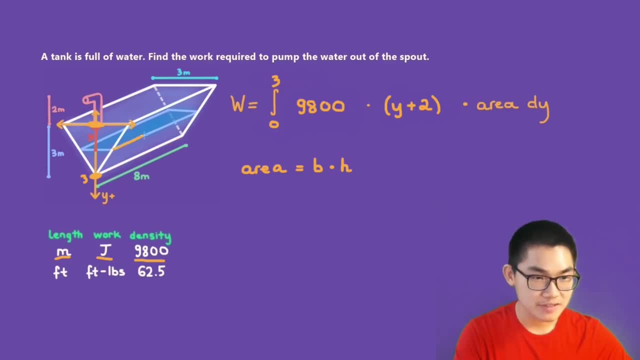 always eight meters. here it's eight, always eight meters. here it's eight meters. as you can see, it is eight meters, meters. as you can see, it is eight meters, meters. as you can see, it is eight meters. so, therefore, this right here will also. so, therefore, this right here will also. 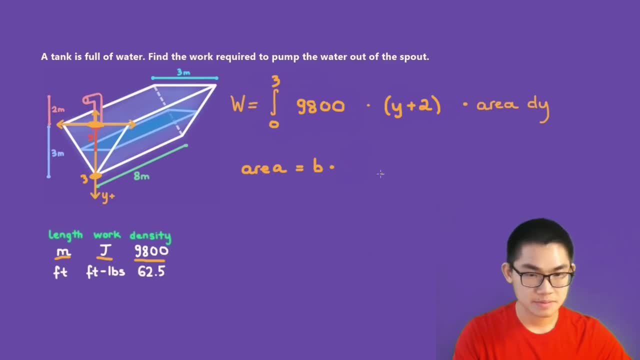 so, therefore, this right here will also be eight meters. and how about the base? and how about the base? and how about the base? well, the base is this distance right? well, the base, is this distance right? well, the base is this distance right. so, first of all, from here to here, this: 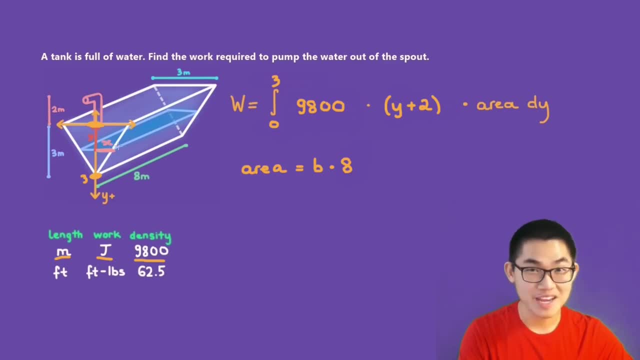 so, first of all, from here to here, this, so, first of all, from here to here this: distance is x, distance is x, distance is x, as explained before in my previous, as explained before in my previous, as explained before in my previous episodes, episodes, episodes. so this means that the base, the complete, 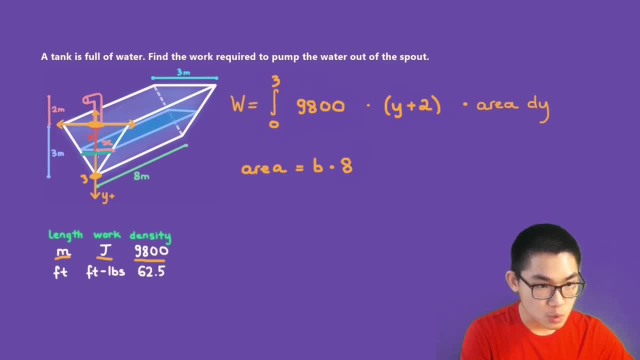 so this means that the base, the complete, so this means that the base, the complete base, base, base from here to here, is 2 times x and because of that, the area is equal to, and because of that, the area is equal to, and because of that, the area is equal to 16x. 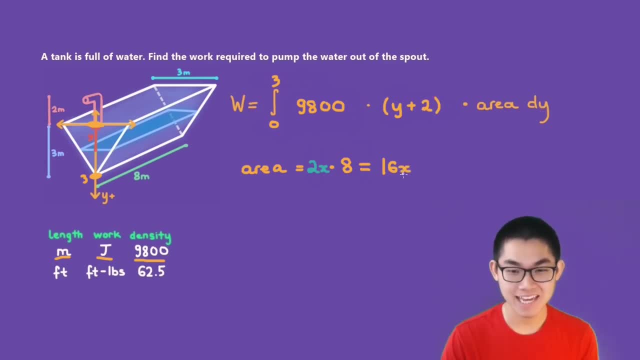 16x, 16x. since our formula is dy, we have to convert. since our formula is dy, we have to convert. since our formula is dy, we have to convert the x, the x, the x into the y- and let me show you how to do- into the y. and let me show you how to do. 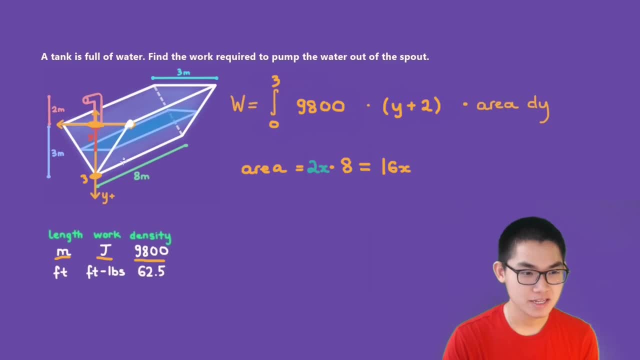 into the y and let me show you how to do that. that, that. so if you look here this point to this, so if you look here this point to this, so if you look here this point to this point, so this is a line right, this point, so this is a line right, this. 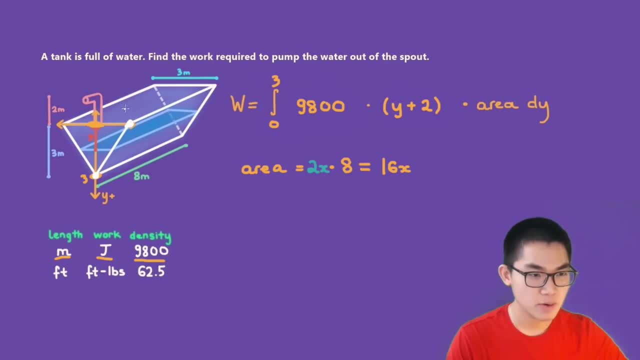 point. so this is a line, right, this right here is a line, and we know that right here is a line, and we know that right here is a line and we know that this point is going to be, this point is going to be, this point is going to be 1.50. 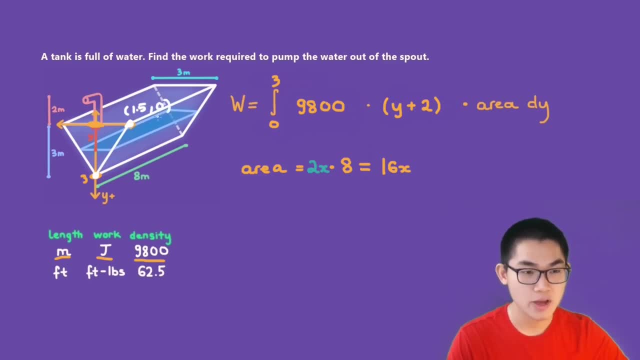 1.50, 1.50. so that point right here is 1.5. so that point right here is 1.5. so that point right here is 1.5, zero. and why is it 1.50? well, because zero. and why is it 1.50? well, because. 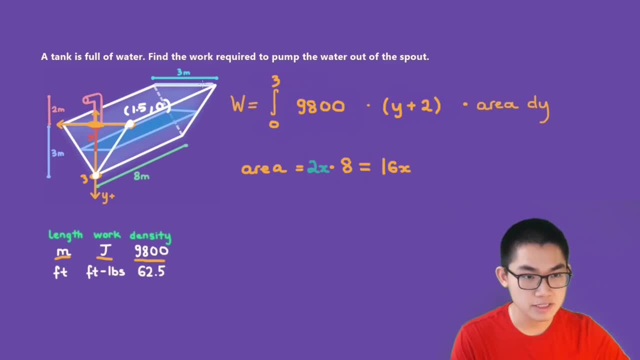 zero. and why is it 1.50? well, because we know that the distance from here to, we know that the distance from here to, we know that the distance from here to here, this distance right here, is three here. this distance right here is three here. this distance right here is three right. so what is half of three? 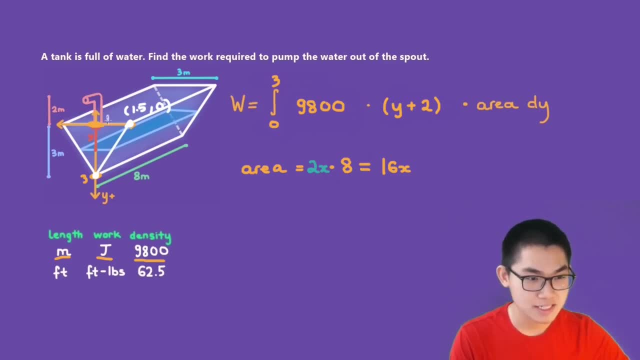 right. so what is half of three? right. so what is half of three? well, half of three is just 1.5. well, half of three is just 1.5. well, half of three is just 1.5, which means that this distance from here. 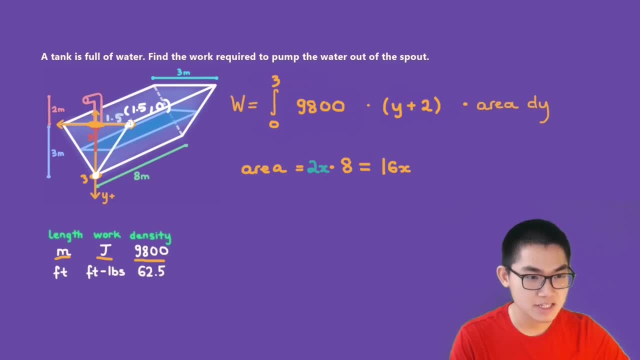 which means that this distance from here, which means that this distance from here to here, to here to here, that is 1.5, and because of that, this, that is 1.5, and because of that, this, that is 1.5, and because of that, this point is 1.50. 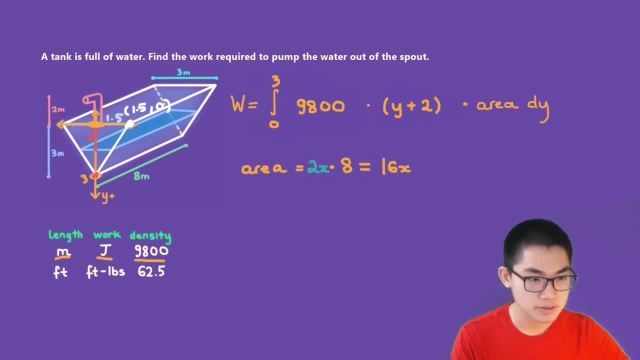 point is 1.50. point is 1.50. now, how about now? how about now? how about? how about this point right here? how about this point right here? how about this point right here? oh, that point would just be. oh, that point would just be. 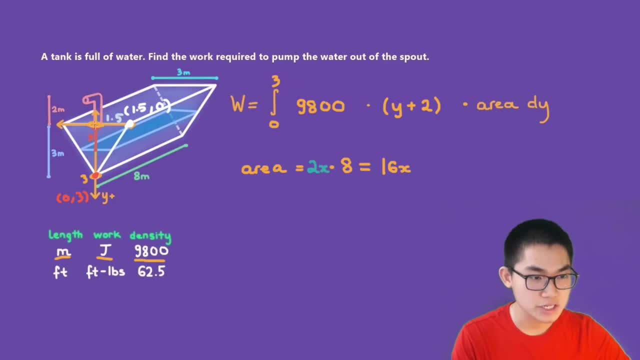 oh, that point would just be zero three, because it is located at the zero three, because it is located at the zero three, because it is located at the origin zero and the height is positive origin zero and the height is positive origin zero and the height is positive three. and notice that three is positive. 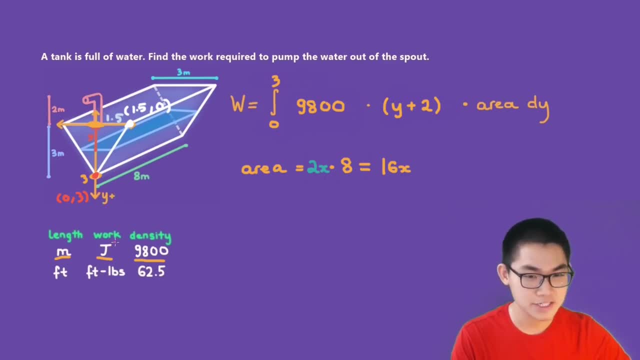 three, and notice that three is positive because we're saying that this direction, because we're saying that this direction, because we're saying that this direction is the positive y direction, is the positive y direction, is the positive y direction. and so let's write down our two points. 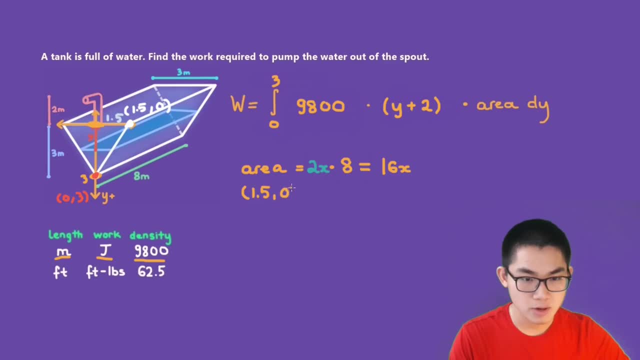 and so let's write down our two points. and so let's write down our two points. we have 1.5, we have 1.5, we have 1.5, 0, and then we also have 0 and 3.. 0, and then we also have 0 and 3.. 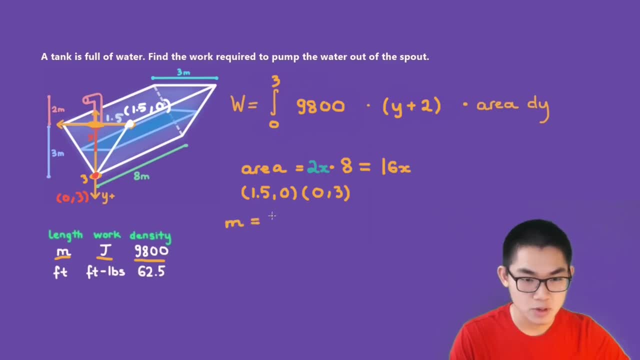 0, and then we also have 0 and 3.. this means that the slope m is equal to. this means that the slope m is equal to. this means that the slope m is equal to 3 minus 0 divided by 0 minus 1.5. 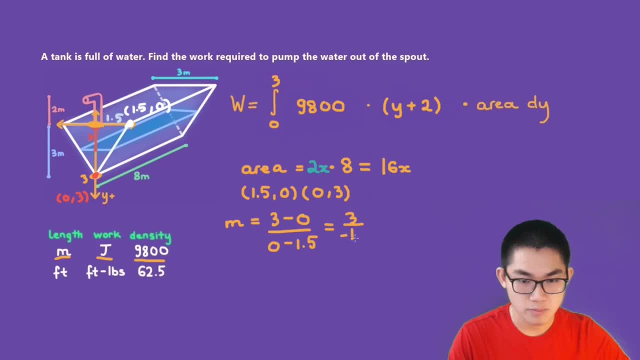 3 minus 0 divided by 0 minus 1.5. 3 minus 0 divided by 0 minus 1.5, this is the same as 3 over negative 1.5. this is the same as 3 over negative 1.5, which is equal to 3 divided by negative. 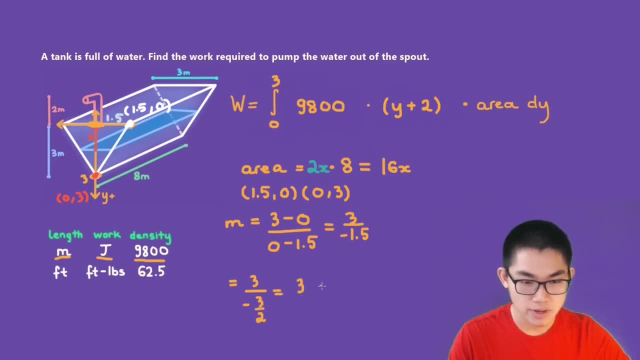 which is equal to 3 divided by negative, which is equal to 3 divided by negative. 3 over 2, and this is the same as 3, 3 over 2, and this is the same as 3, 3 over 2, and this is the same as 3 multiplied by negative: 2 over 3. 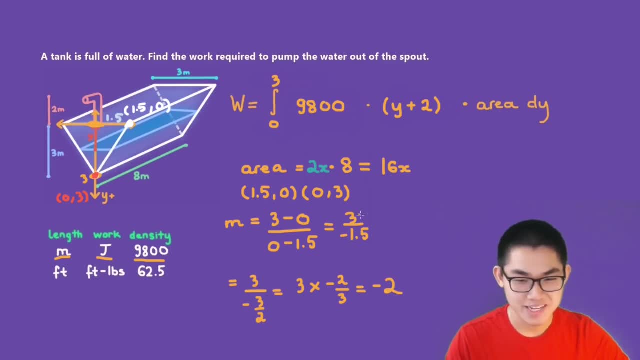 multiplied by negative 2 over 3, multiplied by negative 2 over 3, which is equal to negative 2, right so, which is equal to negative 2, right so, which is equal to negative 2, right so this right here is equal to negative 2. 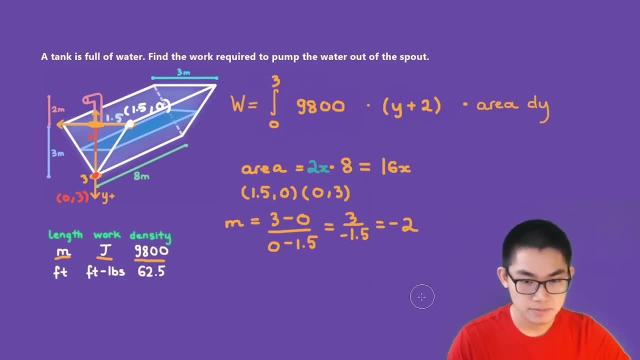 this right here is equal to negative 2. this right here is equal to negative 2, and let's go ahead and erase this right, and let's go ahead and erase this right, and let's go ahead and erase this right here, here. here, our point slope formula will be: y is. 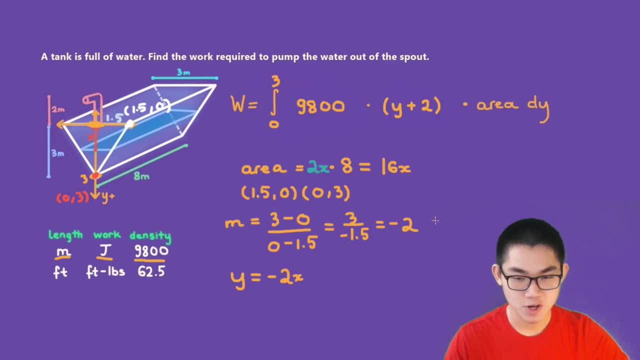 our point slope formula will be: y is. our point slope formula will be: y is equal to negative x, equal to negative x, equal to negative x, which is the slope that we found, which is the slope that we found, which is the slope that we found plus b. 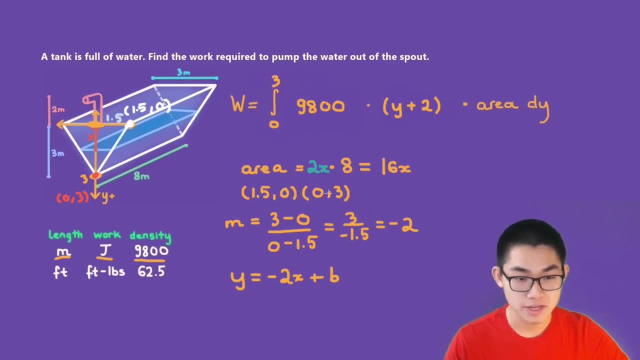 plus b plus b, and all we have to do is substitute one, and all we have to do is substitute one, and all we have to do is substitute one over these two points in here, over these two points in here, over these two points in here, and i'm going to substitute this point. 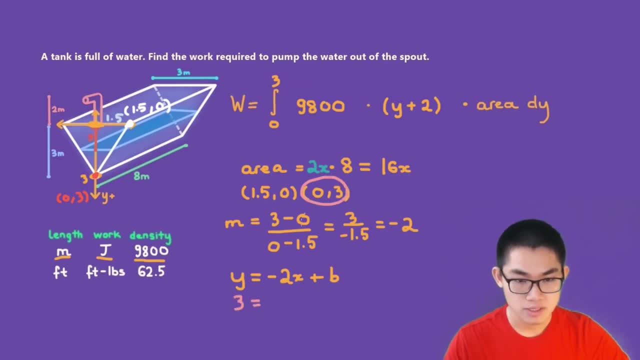 and i'm going to substitute this point. and i'm going to substitute this point. so y is equal to 3, so y is equal to 3, so y is equal to 3, is equal to, is equal to, is equal to negative 2 times x, and x is 0, right? so? 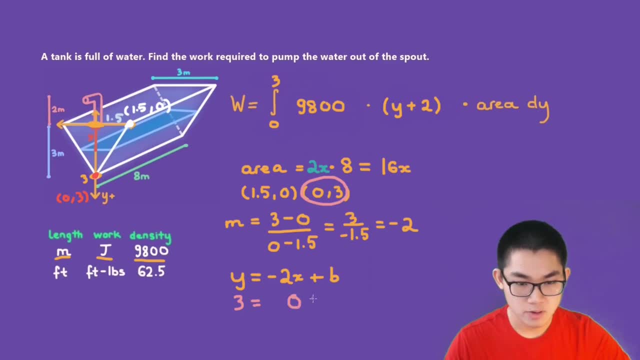 negative 2 times x and x is 0, right, so negative 2 times x and x is 0, right so this times 0, which just means that this this times 0, which just means that this this times 0, which just means that this, right here, is 0. 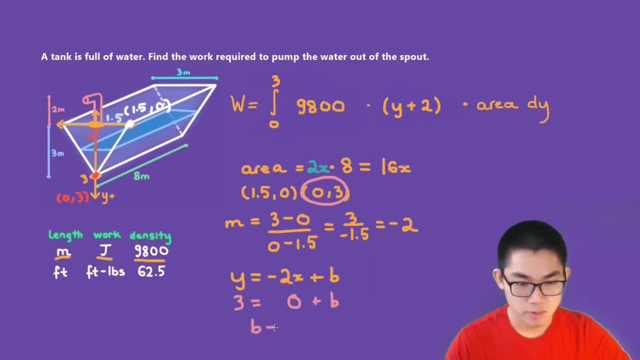 right here is 0, right here is 0 plus b, so b is equal to 3. so let's delete the b and write number. so let's delete the b and write number. so let's delete the b and write number. 3 right here. 3 right here. 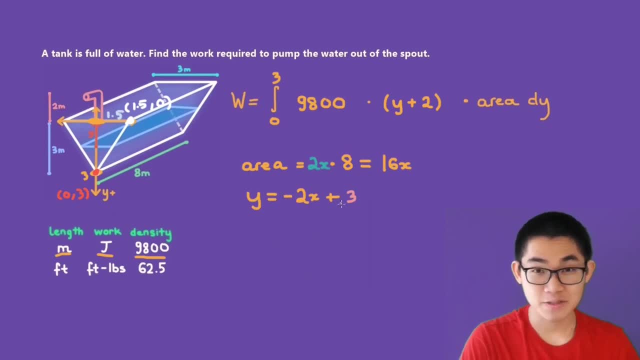 3, right here. our equation is: y is equal to negative. our equation is: y is equal to negative. our equation is: y is equal to negative. 2x plus 3 and we're going to solve for 2x plus 3 and we're going to solve for. 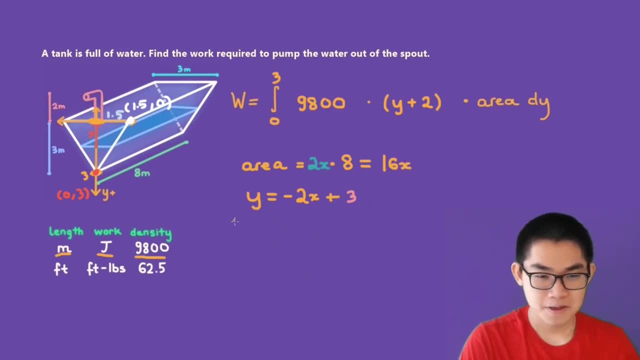 2x plus 3 and we're going to solve for x, so we can put it back into our area x. so we can put it back into our area x. so we can put it back into our area formula, formula, formula. so we get y plus 2x. y plus 2x is: 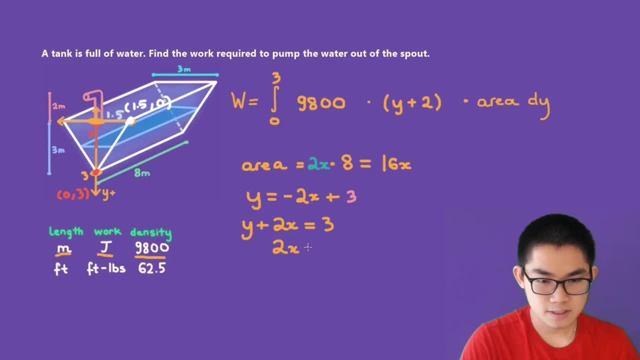 so we get y plus 2x. y plus 2x is, so we get y plus 2x. y plus 2x is equal to 3 minus y, equal to 3 minus y, equal to 3 minus y. so x is equal to 1 over 2. 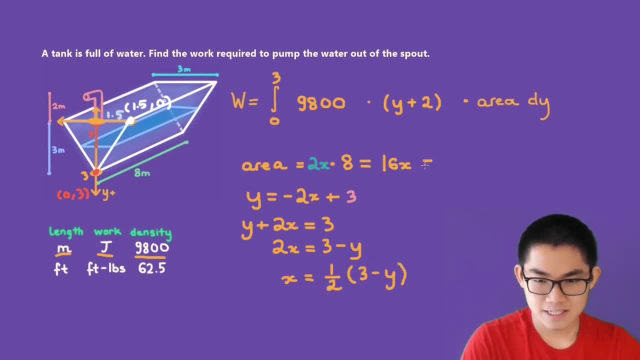 so x is equal to 1 over 2. so x is equal to 1 over 2 times 3 minus y times 3 minus y times 3 minus y, 16x is the same as 16. 16x is the same as 16. 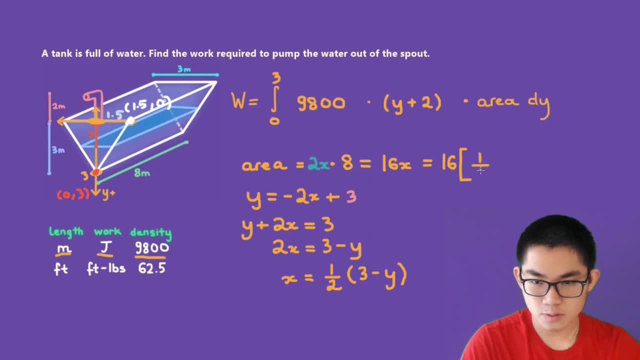 16x is the same as 16 times x, which is 1 over 2, 1 over 2 times x, which is 1 over 2, 1 over 2 times x, which is 1 over 2, 1 over 2 times 3 minus y. 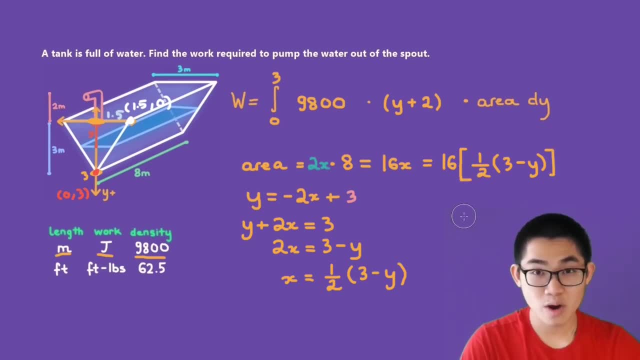 times 3 minus y, times 3 minus y, and we can close the bracket and we can close the bracket and we can close the bracket. 16 times 1 over 2 is the same as 8. 16 times 1 over 2 is the same as 8. 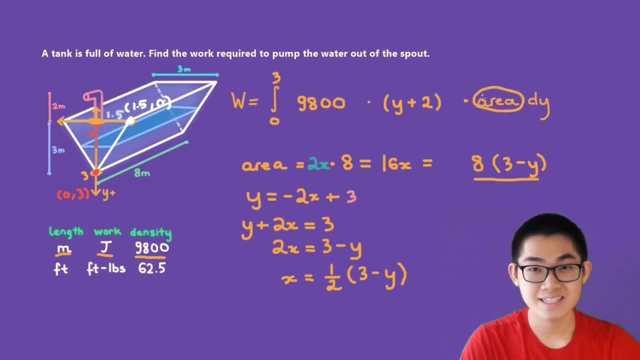 16 times 1 over 2 is the same as 8. let's go ahead and put this into our. let's go ahead and put this into our. let's go ahead and put this into our area, area, area. the last step is to evaluate this. 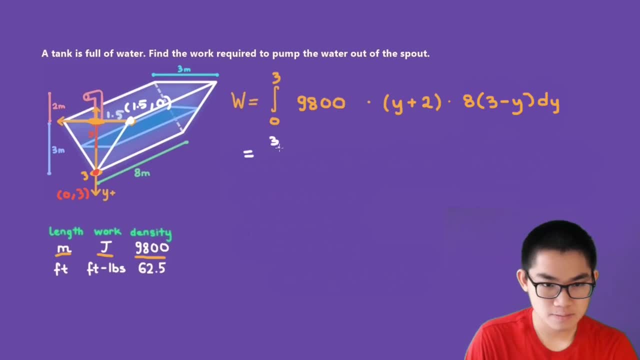 the last step is to evaluate this. the last step is to evaluate this integral. this is equal to the integral integral. this is equal to the integral integral. this is equal to the integral from 0 to 3, from 0 to 3, from 0 to 3, and then 9 800 times 8 will give you. 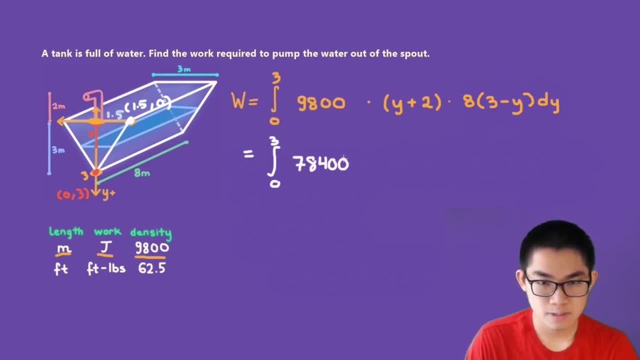 and then 9 800 times 8 will give you, and then 9 800 times 8 will give you 78 400, 78 400, 78 400, and then times y plus 2, and then times y plus 2, and then times y plus 2 times 3 minus y. and don't forget the dy. 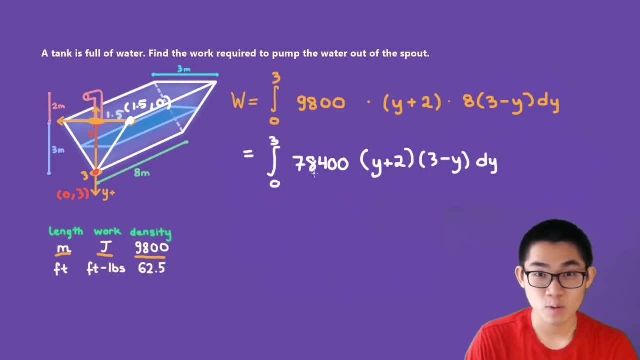 times 3 minus y, and don't forget the dy, times 3 minus y, and don't forget the dy. since 78 400 is a constant, we can move. since 78 400 is a constant, we can move. since 78 400 is a constant, we can move it outside of the integral. 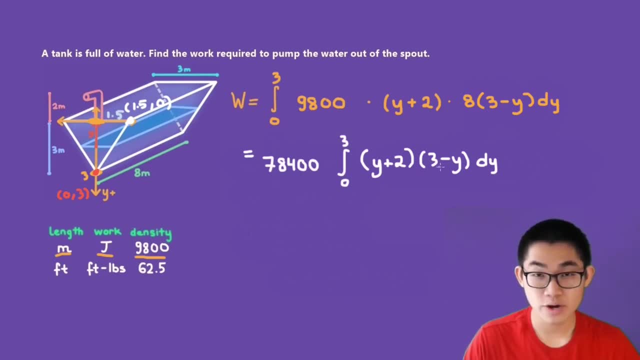 it outside of the integral. it outside of the integral. now, what is y plus 2 times 3 minus y? now, what is y plus 2 times 3 minus y? now what is y plus 2 times 3 minus y? let's find out. we have y. 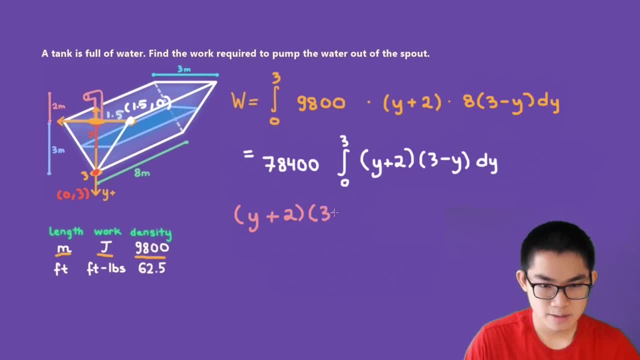 let's find out: we have y. let's find out: we have: y plus 2 times plus 2 times plus 2 times 3 minus y 3 minus y. 3 minus y. y times 3 gives us 3y, y times 3 gives us 3y. 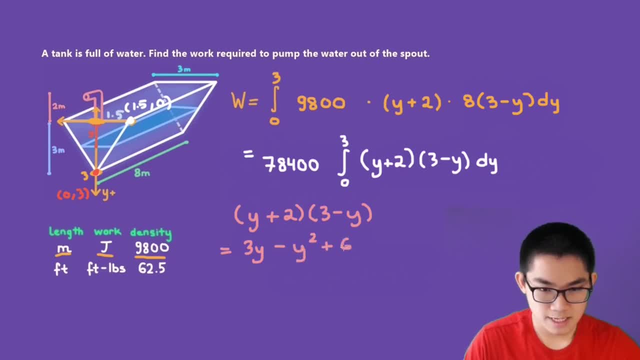 y times 3 gives us 3y minus y to the power of 2 minus y to the power of 2 minus y to the power of 2 plus 6 minus 2y plus 6 minus 2y plus 6 minus 2y. this is the same as negative y square. 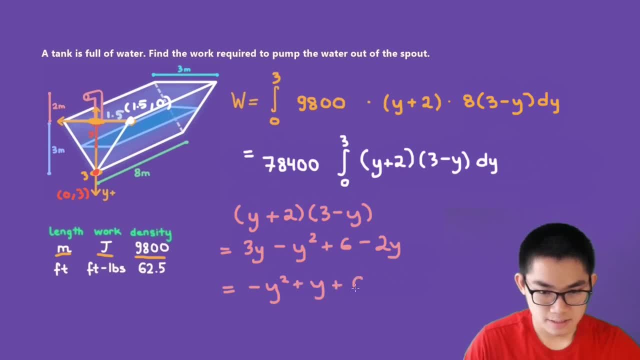 this is the same as negative y square. this is the same as negative y square plus y plus y plus 6. after I solve this integral, I got 1, 0, 5, 8, 4, 0, 0. so if you solve this, this is the number that you should also get, and the unit is going to be in Joules. so 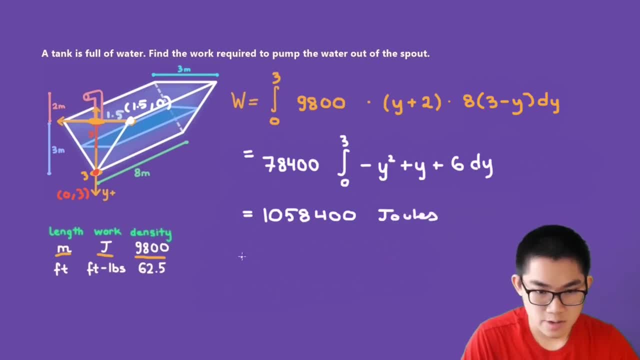 this was going to be Joules, and you can also approximate this into 1.06 times 10, to the power of 6 Joules. so this right here is the answer, and also the amount of work that it takes to pump all of the layers of water out of. 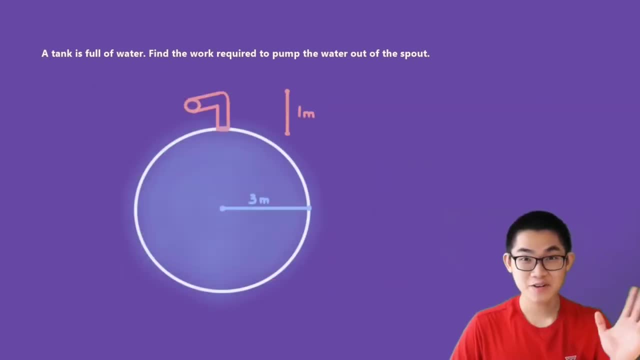 the tank and also out of the spout. hi everyone, in this video I'm gonna show you how to calculate the amount of work that it takes to pump all the water out of this three-dimensional sphere. so we're given a tank. this tank is full of. water and we're going to calculate the amount of water that it takes to pump all of the layers of water out of the spout. hi everyone, in this video I'm gonna show you how to calculate the amount of work that it takes to pump all the layers of. 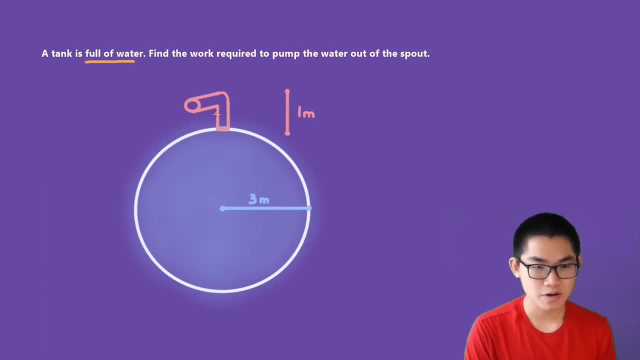 water and we have to find the amount of work to pump all of this water out of the spout. so the radius of this circle, or rather this three-dimensional sphere, is 3 meters. that's the radius, and we also know that the height of the spout. 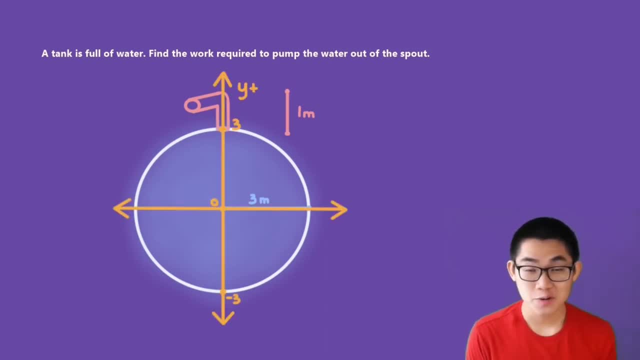 is 1 meter for a circle. what you want to do is put the X and Y axis at the center, so this time the origin is at the center and the positive y direction is upwards. okay, so don't forget that. to empty this tank, all we have to do 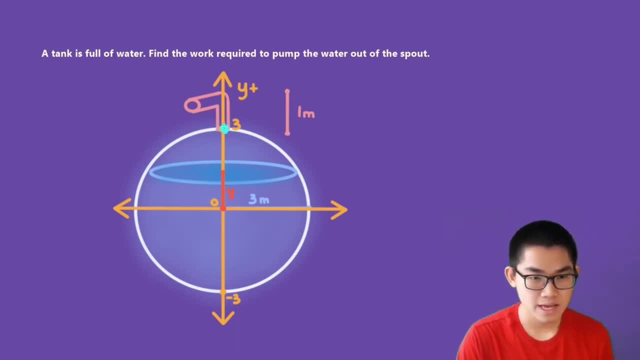 is move every single layer of water from here to here. right, so this is just one layer of water, but you can imagine that there are many, many layers of water in here, just like this one, and we want to move it to the top. so we're going to move this to the top of the tank now. one thing to notice is: 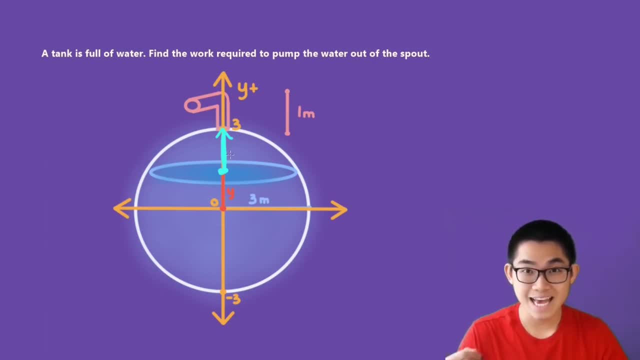 that in our previous episodes, we have already established the fact that the distance from the origin to our layer of water is y. so what is this distance? well, this distance will simply be 3 minus y, and that's because the radius is 3. the radius is 3, which means from here to here. 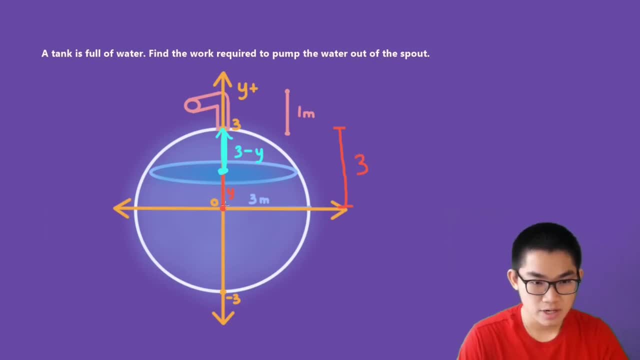 is 3, the radius is 3 and we know that this is y. so the blue, the blue, the blue distance, the blue distance right here, must be 3 minus y. so, like i said, this distance will be 3 minus y and our diagram is finished. we are prepared and ready to solve this problem. to calculate the 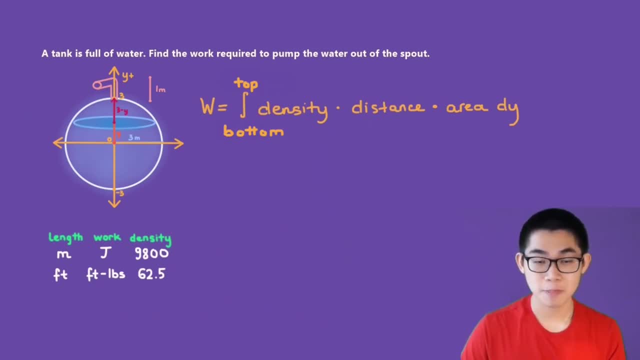 work. we're going to use the formula that we have been using, but the only difference is that, because the positive y direction is pointing upwards, this time the bottom will be down here and the top will be up here. okay, so that's the only difference. so work will be equal to the integral from. 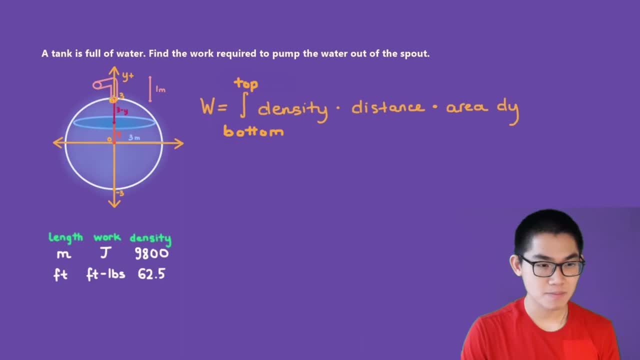 the bottom to the top of density, times, distance times, area. so what is the top and what is the bottom? well, as mentioned before, we want to empty the tank from here to here, right, in order to empty the whole thing. so the top will be 3 and the bottom will be minus 3. 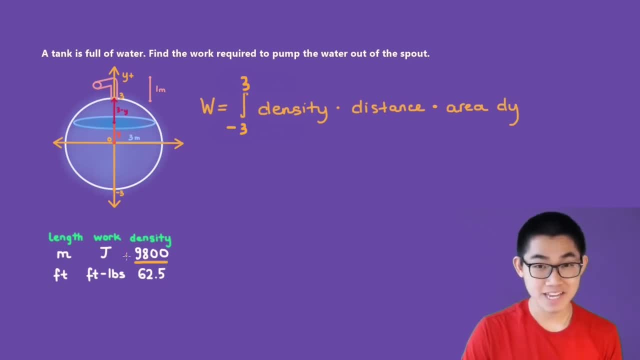 9,800, right, according to our table, because the length given is in meters, and so our work will be in joules. as for the distance removing each layer of water to the top, right, we're moving from here to here, to the top, and the distance that we're moving to the top is. 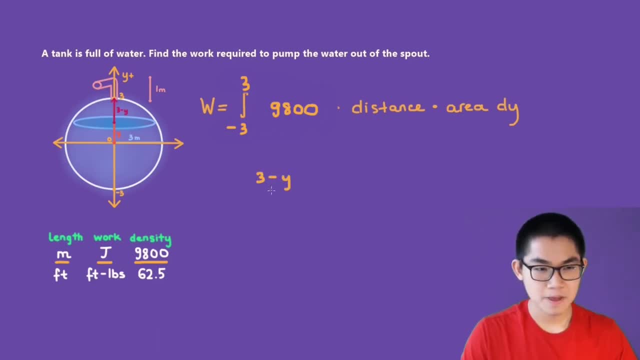 three minus Y. but don't forget, we're also moving it outside of the spout. so we have to move it out of the spout. and we know that the height of the spout is one meter, so we have to plus one, and this is the same as. 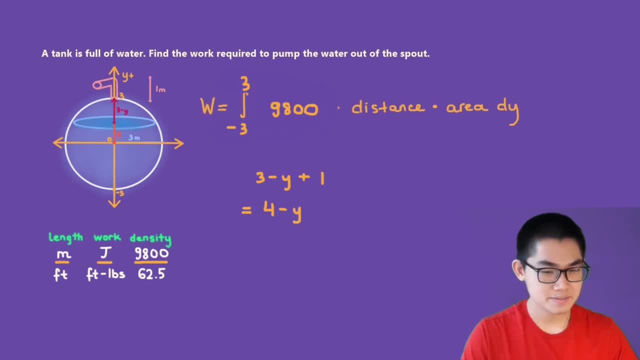 four minus Y. how about the area? well, the area of our layer of water. so that area is equal to I radius, to the power of two, and the radius is from here to here, and we can also call it X. so instead of writing R, I'm going to write it in terms of X. you 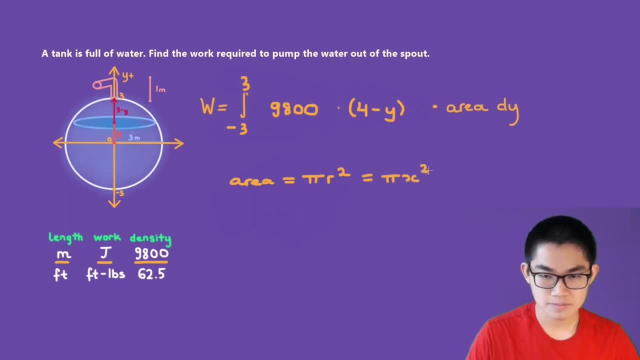 get pi times X to the power of two. since our formula is dy, we have to convert the X into a Y, and let me show you how to do that. we know that the equation of this entire circle, so the equation of that entire circle, is Y to the power of two plus X to the power of two, is equal to three to the.